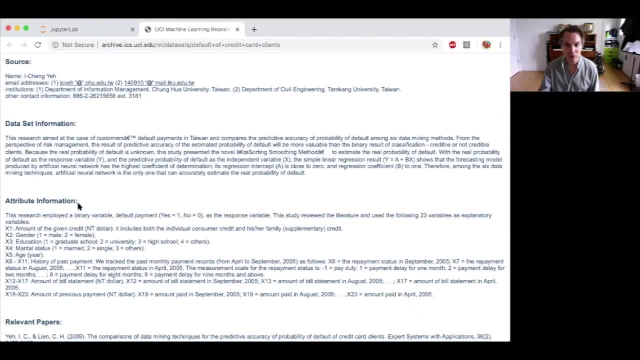 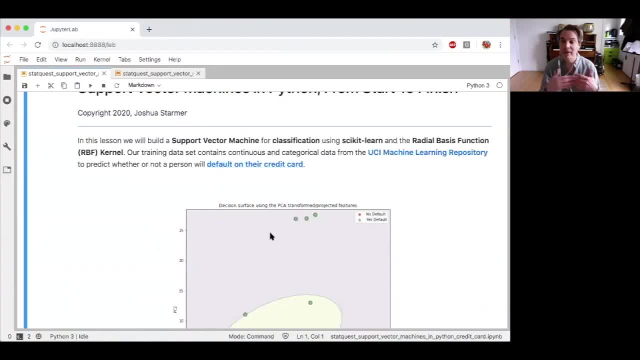 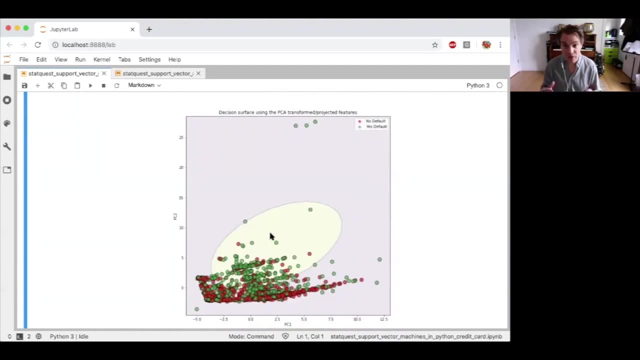 Just click on the link and there it is, and you see we've got attribute information that describes the data and the data set, And so there's lots of sort of stuff you can click on and learn more about. Here is a picture of the decision surface that we will create with our support vector machine. We'll do this at the end, But I just want to give you a sneak preview of what's going to happen. 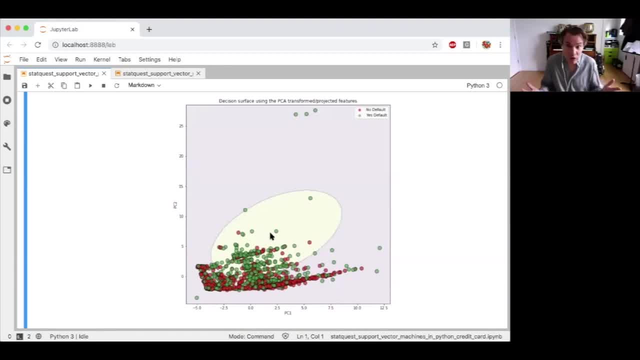 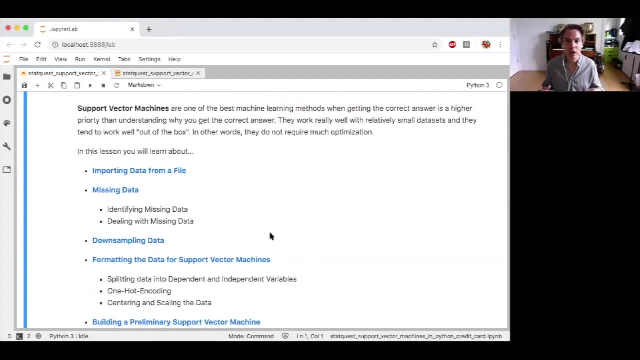 It's kind of a messy figure, but it's what we're going to do, So let's just Let's move on. Okay, so support vector machines. why would you wanna do them? They are one of the best machine learning algorithms out there. for when getting the correct answer. 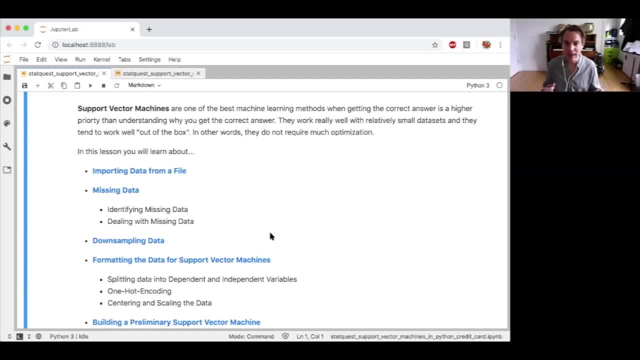 is a higher priority than actually understanding why you get the correct answer. They work really well with relatively small data sets and they tend to work well out of the box. In other words, they tend to not require much optimization. So in this lesson we're gonna learn: 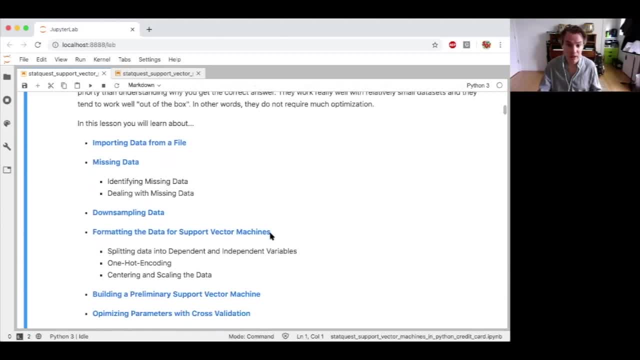 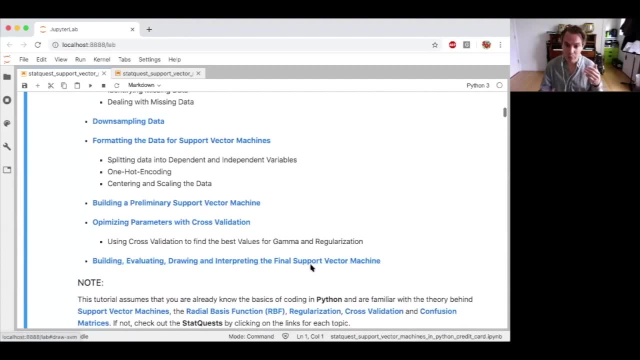 about importing data from a file. We're gonna learn about missing data, down, sampling data, formatting the data for support vector machines, and we're gonna build a preliminary support vector machine. Then we're gonna optimize it and then we're gonna build evaluate draw. 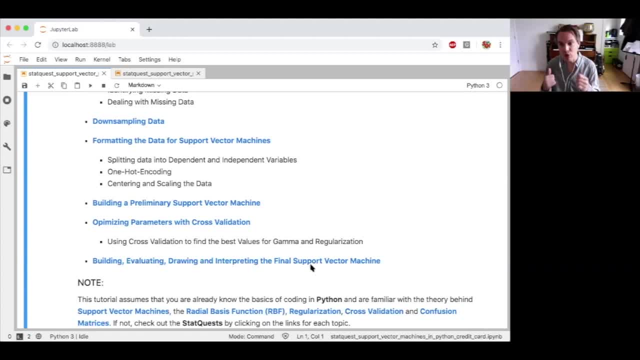 and interpret a final support vector machine and we're gonna compare it to that preliminary machine And we're gonna see if it does better or it doesn't do better. One of the things about support vector machines is because they're great out of the box. 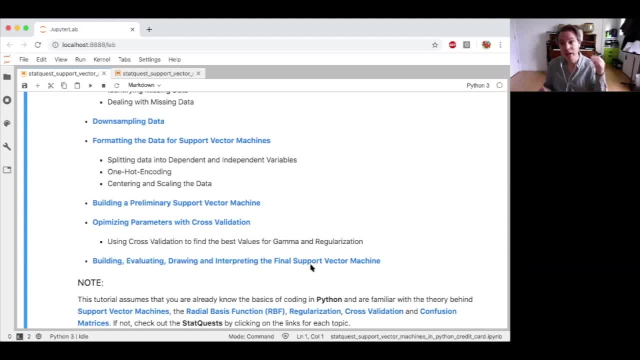 sometimes optimizing doesn't give you a huge bonus, like when you're using classification trees. When we did that, it was night and day. It was like we went from a huge tree to a prune tree and that prune tree was infinitely better at doing classification. 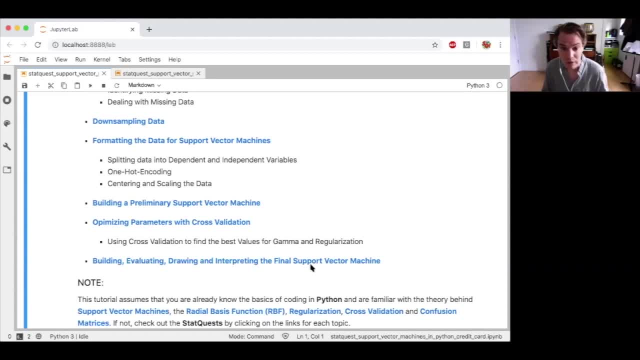 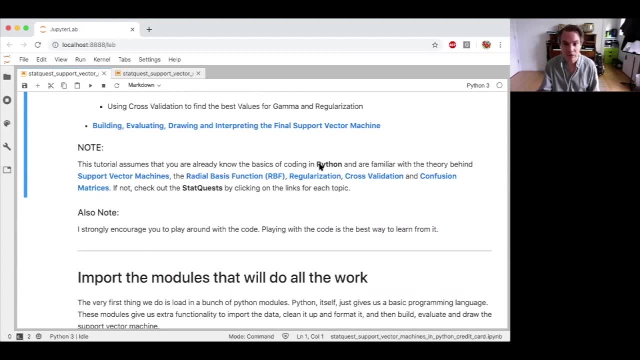 In contrast, support vector machines tend to be pretty good out of the box, So let's just see what happens. Note: this tutorial assumes that you already know the basics of Python and are familiar with the theory behind support vector machines: the radial basis function regularization. 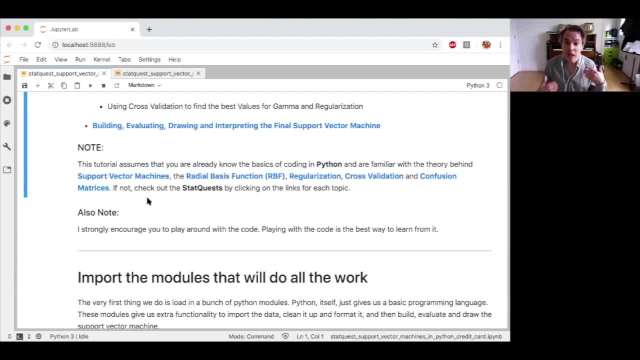 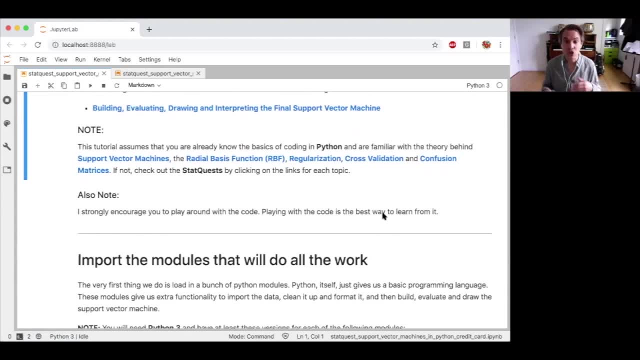 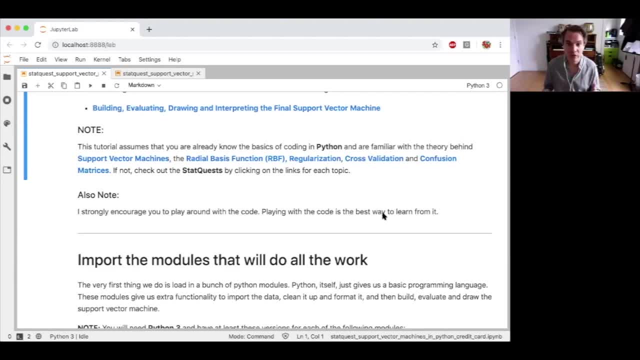 Playing with code is the best way to learn from it. There's alternative ways to do what we wanna do in this Jupyter notebook and there are different ways to optimize. and there's different ways. you can even just plug in different machine learning algorithms. 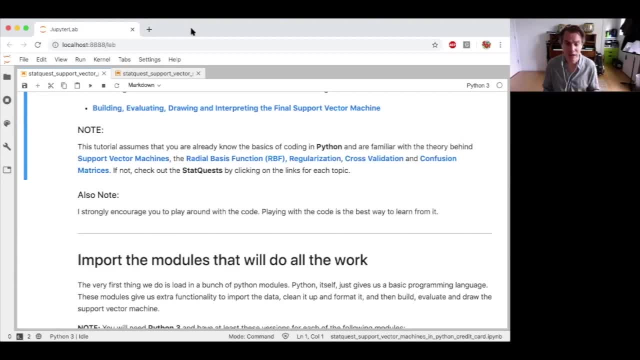 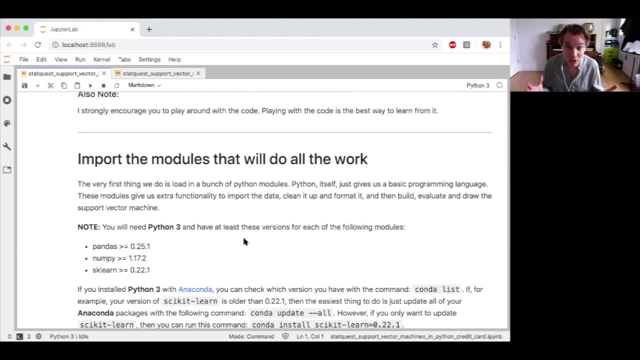 for that matter, and just see what happens. There's a lot of learning that can take place by just playing around, And that's when I think that's the exciting part. I mean, this is pretty fun too, so don't get me wrong. 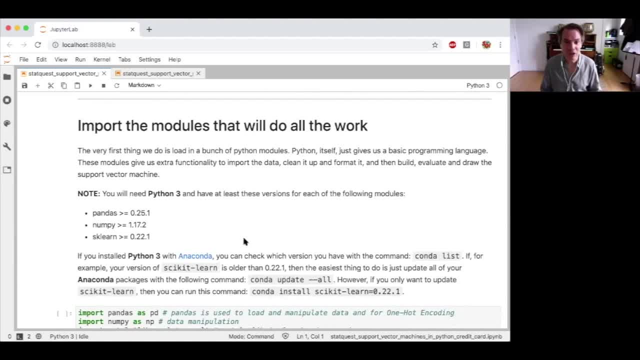 Okay, so the very first thing we're gonna do is we're gonna import the modules that will do all the work. Python itself just gives us a basic programming language. These modules give us extra functionality to import the data, clean it up and format it. 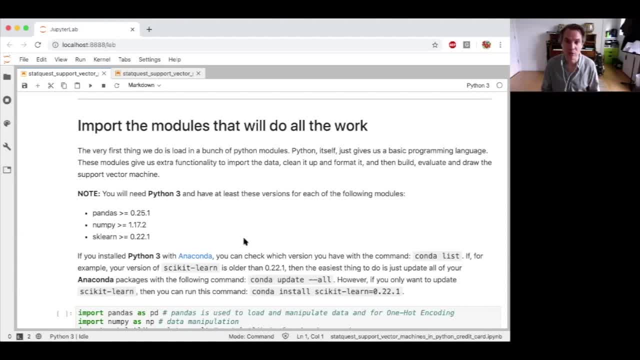 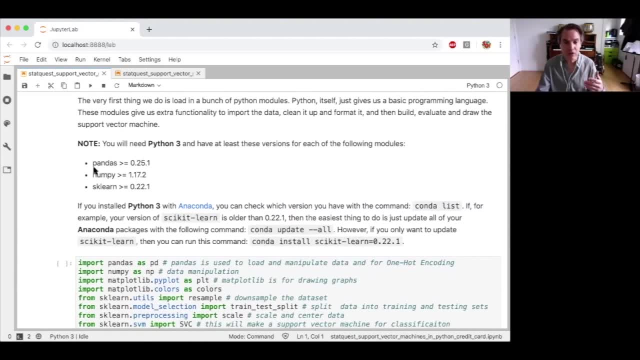 and then build, evaluate and draw the support vector machine. Note: you're gonna need Python 3, and I've got instructions on how to install that and make sure all your modules are up to date down here. We don't need to go through that. 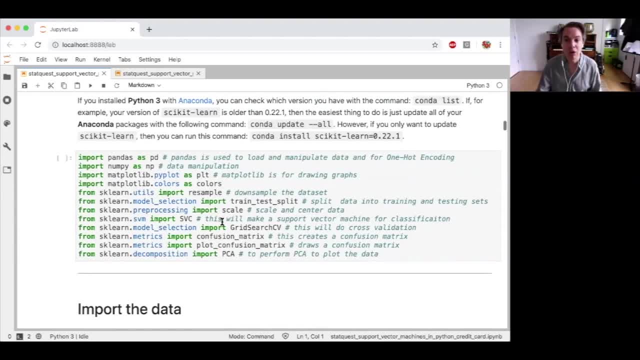 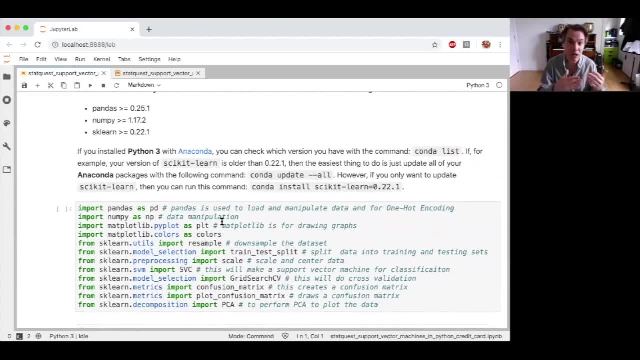 because I've already got this set up on my own computer. However, I do wanna say that we're using a Jupyter notebook and, as you can see, Jupyter notebooks are a nice way to combine text with code, And so here is some code. 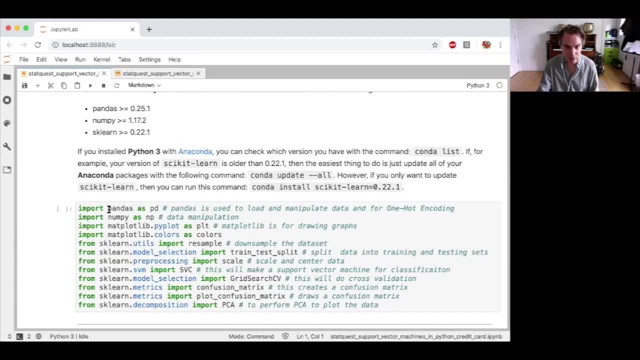 This is where we're importing the modules. We're importing pandas to load and manipulate the data and we're using it for one-hot encoding. There's also Num NumPy that we're gonna use for data manipulation. We're importing matplotlib for graphs. 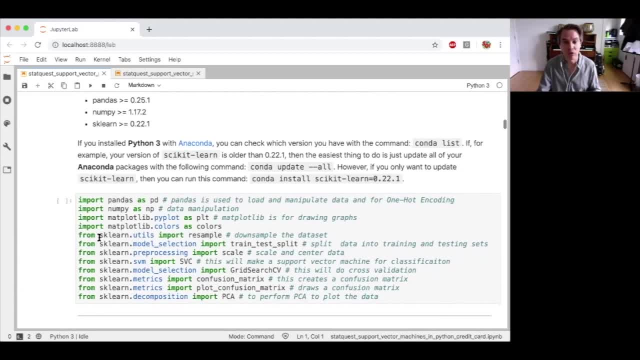 and making things look cool, And we're also importing a lot of scikit-learn stuff to do support vector machines and do confusion matrices and whatnot. Now, when you have a Jupyter notebook, the way you run the code is you click somewhere. 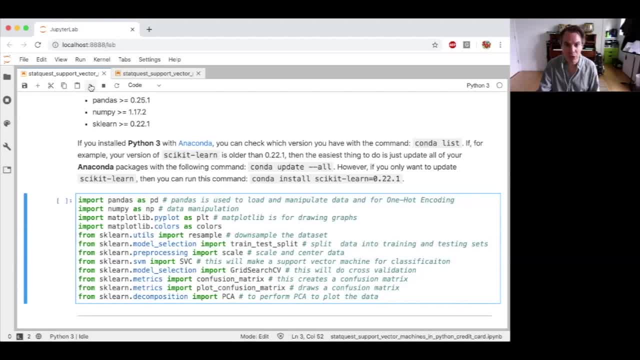 in that block of code and you can either click on this play button up here to run the code. There's a run menu and you can say run selected cells. or on your computer there's a key combination. On a Macintosh it's command enter or control enter. 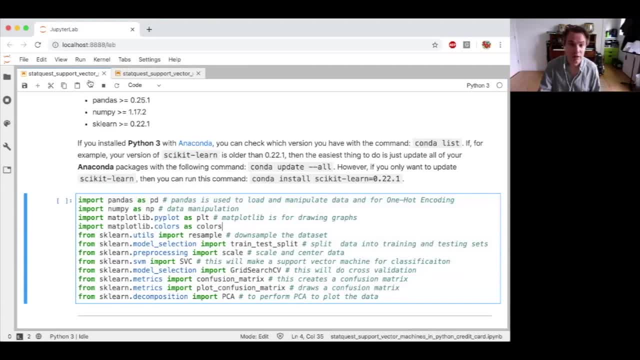 On different computer systems it's different. So just click the run menu and it'll tell you what to do. So what I'm gonna do is I'm gonna click in this block of code and we're gonna run it, And when you run it briefly, you might have missed it. 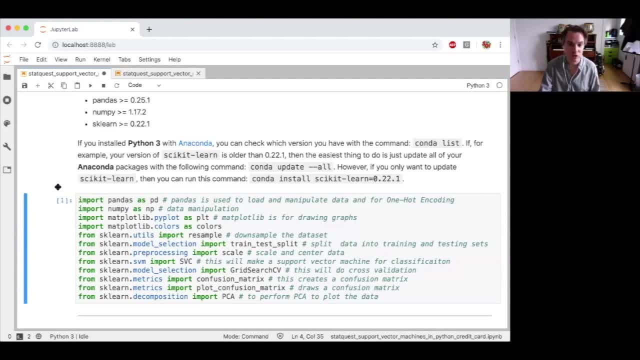 There was a star there before it turned into a number one. The star means that Python is doing something and at that time it was loading the modules, And when it gives you a number, that means it's done, doing whatever it was doing. 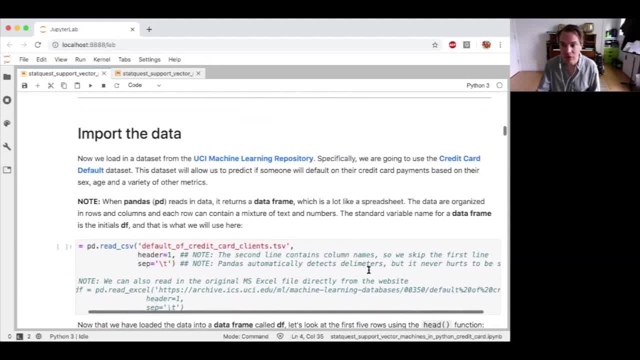 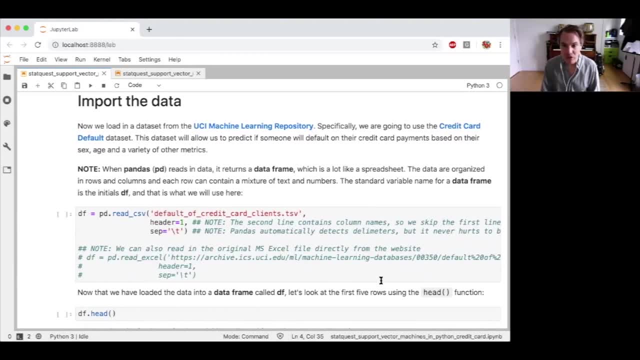 So it loaded the modules pretty quickly. Okay, now we're ready to import the data. Now we load the data set From the UCI machine learning repository. Specifically, we are going to use the credit card default data set. This data set will allow us to predict. 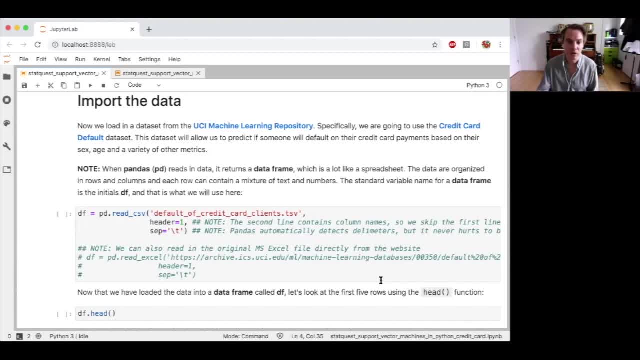 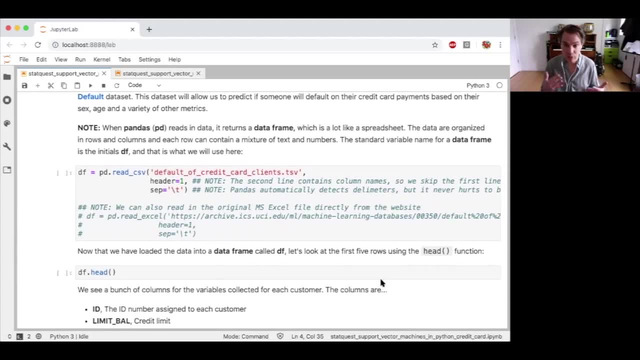 if someone will default on their credit card payments based on their sex, age and a variety of other metrics. Note when pandas, which is what we're gonna use to read in the data. when it reads in data, it returns a data frame which is a lot like a spreadsheet. 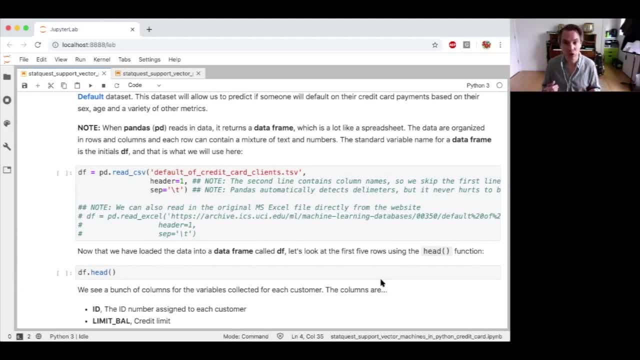 The data are organized in rows and columns, and each row can contain a mixture of text and columns- Excuse me- text and numbers. The standard variable name for a data frame is the initials df, and that's what we're gonna use here. 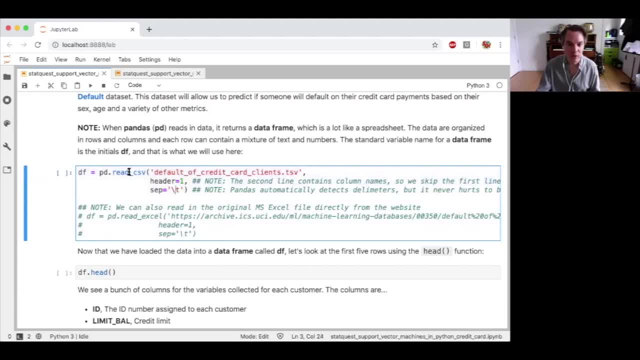 And I've got two blocks of code here. One is to read in the file that we're gonna use. This is a file that will be included with the Jupyter notebook, so you don't have to download it or anything. We're gonna be using read underscore CSV to read it in. 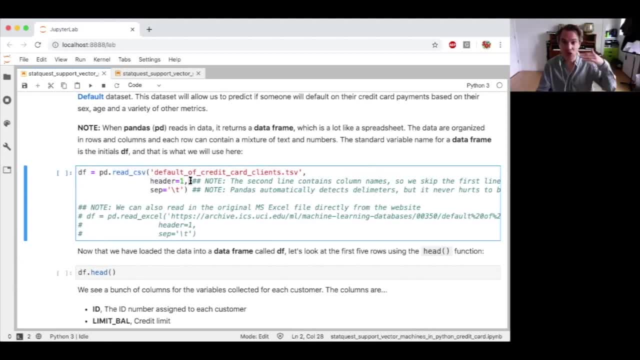 The file has a header row, so the very first row- actually it's the second row in the data set- has the header information. The first row has some other kind of nonsense and I don't actually remember what it was And it's tab delimited. so we're setting the separator. 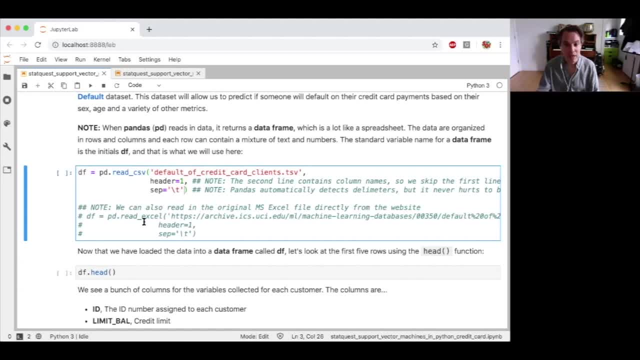 to the tab escape sequence. However, you can also read this directly from the UCI machine learning repository directly. You don't have to download the file first And this is commented out so it won't be running, but when you play around with the code later. 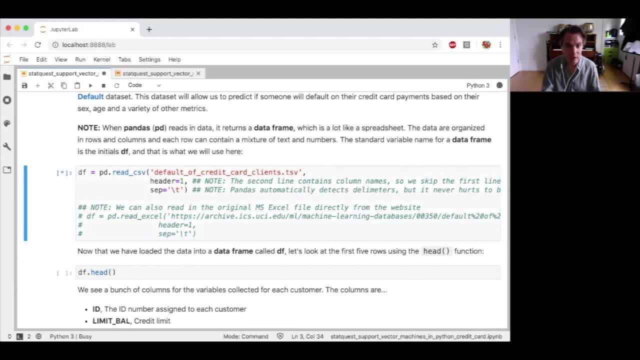 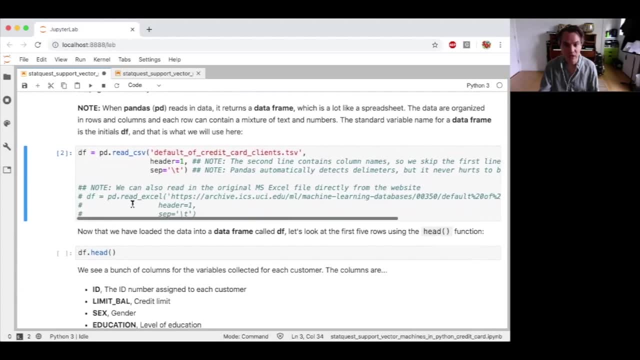 you can feel free to play with it yourself. Okay, so we'll load in the data and there we are. We've got a number here. That means we ran the code, And so, now that we've loaded the data into a data frame called df- 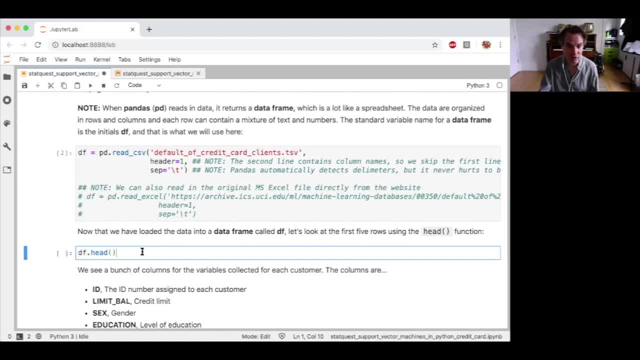 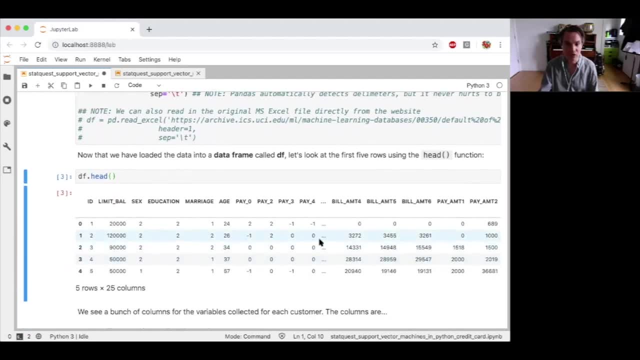 we're gonna look at the first five rows using the head function, So let's just run that. So we've got dfhead and that returns us the first five rows And we see that we have a bunch of columns for the variables collected for each customer. 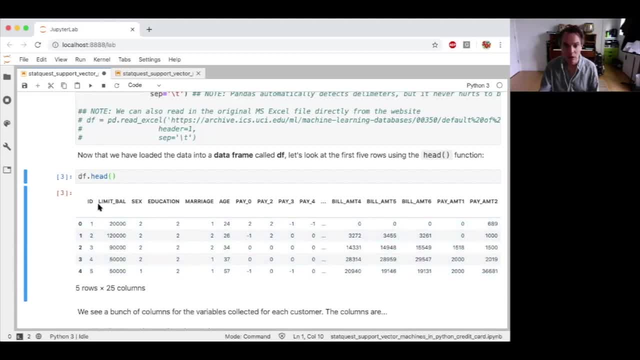 The columns are ID, that's just an ID number. A limit balance is the credit limit for that customer. Sex is male or female. Education, marriage, age, payment. These columns tell us whether or not the last payment was on time or later, or how long. 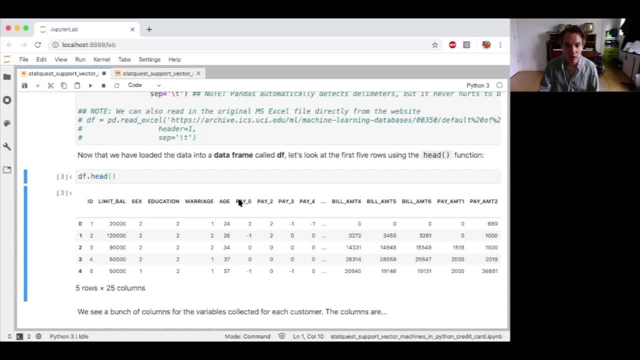 Or how late it was. There's one column for different months of payments, So it's not just one last month's payment, It goes back six months. Then we have the bill amounts for the last six months, the last six bills and how much was paid for the last six bills. 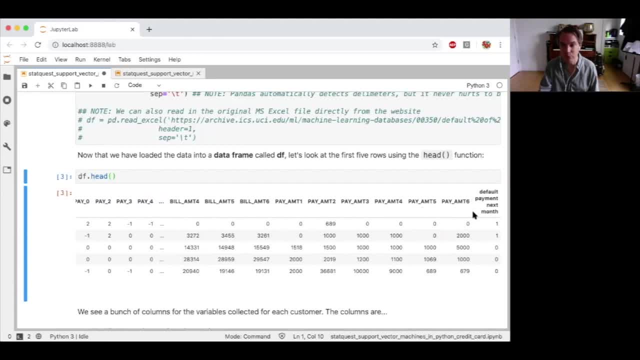 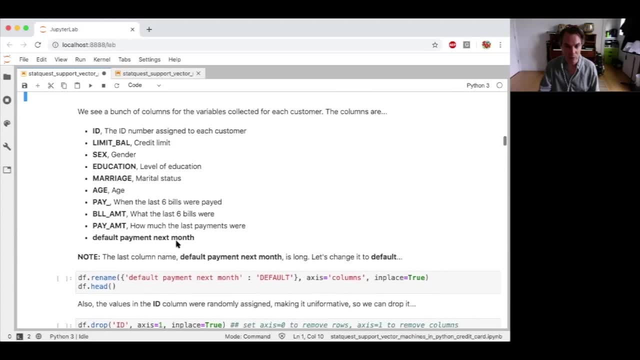 And then, lastly, we have default payment next month. This is the variable that we're going to try to produce, So we're going to call it default payment next month, And then we're going to change it to just be default, And here I've listed the column names as well. 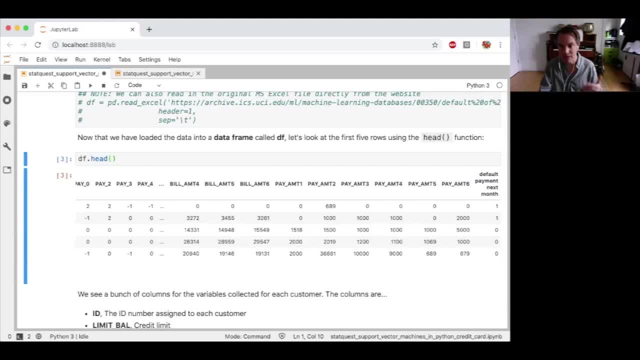 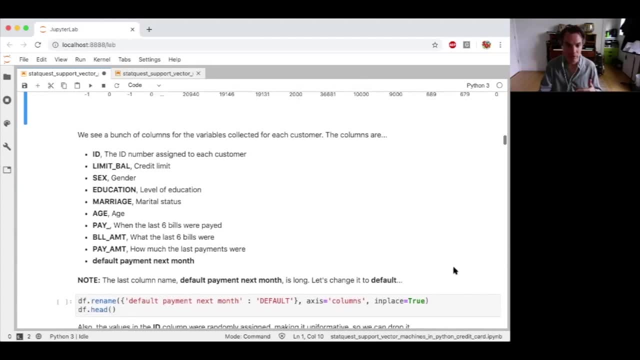 But note the last column name, this one default payment next month. that is a mouthful, So we're going to change it to just be default. So did they default or not? And we do that by doing dataframerename And we pass in the column name that we want to change and then 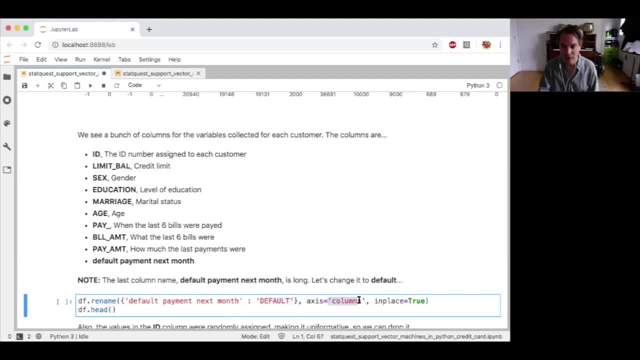 the name we want to change it to. We set access to columns. We're specifying that we want to change a column name. Lastly, we're saying we want to do it in place, meaning we're going to modify this dataframe. We're not going to make it copy and then save it as a new variable. 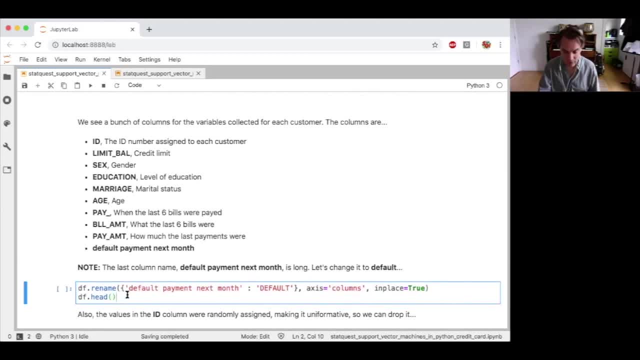 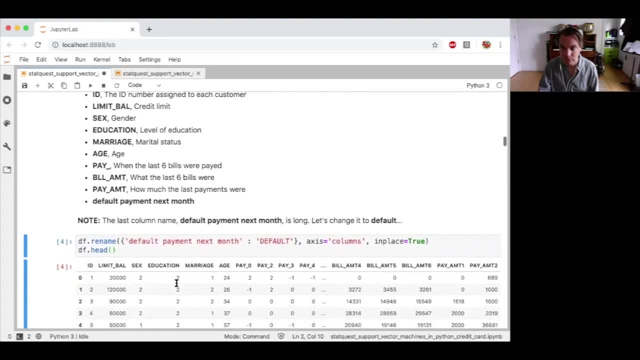 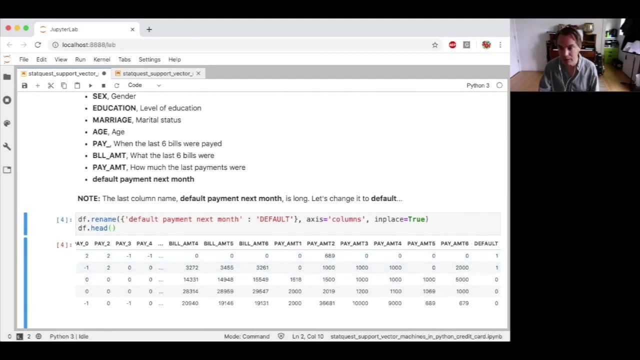 And then what we're going to do is we're going to print out the first five rows and we're going to verify that we renamed the column correctly. Okay, So we look over here and we see that the last column name is now default. 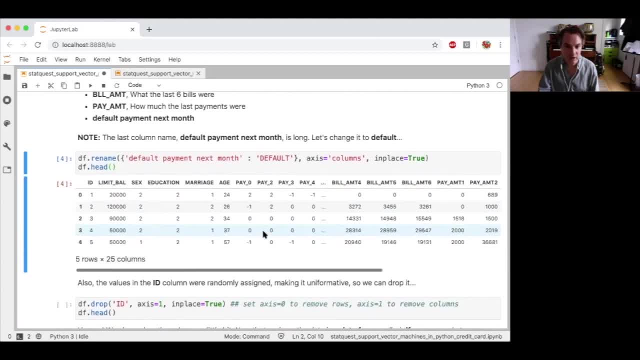 And that's great. That's what we wanted. The other thing is this ID column. These are just random numbers that were assigned to each customer and they're not informative, so we're going to drop it. So we'll do that with dfdrop and we're specifying the ID column. 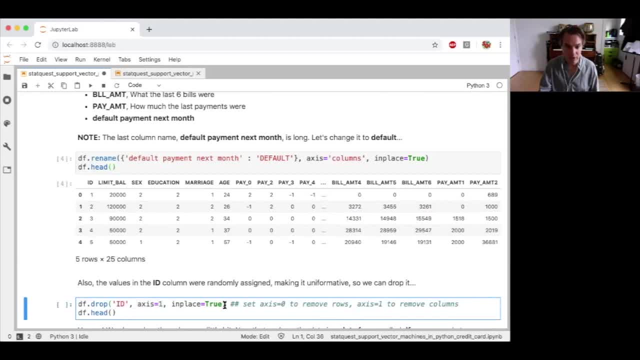 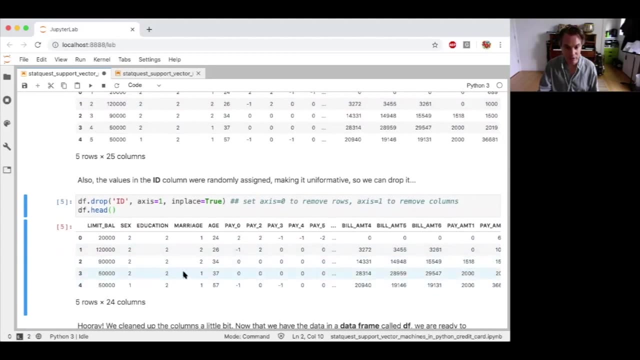 Again, this is a column And we're going to do this in place, just like we did before, and we're going to print out the first five rows to verify that. we removed the column And there it is, Like we've got ID up here and now we no longer have the ID. 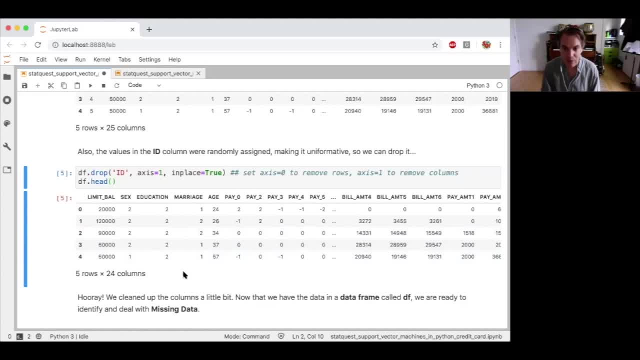 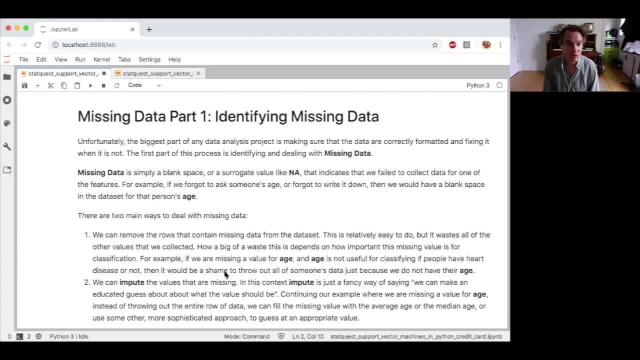 So, hooray, We've cleaned up the columns a bit and now that we have the data in a dataframe called df, we are ready to identify and deal with missing data. Unfortunately, the biggest part of any data analysis project is making sure that the data are correctly formatted. 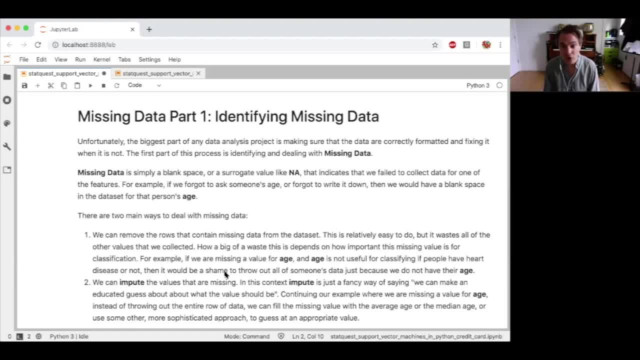 and fixing it when it is not. The first part of this process is identifying and dealing with missing data. Missing data is simply a blank space or a surrogate value like NA that indicates that we failed to collect data for one of the features, For example, if we forgot to ask someone's age or forgot to write it down. 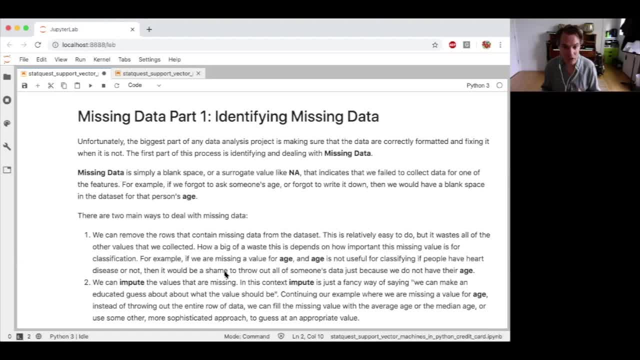 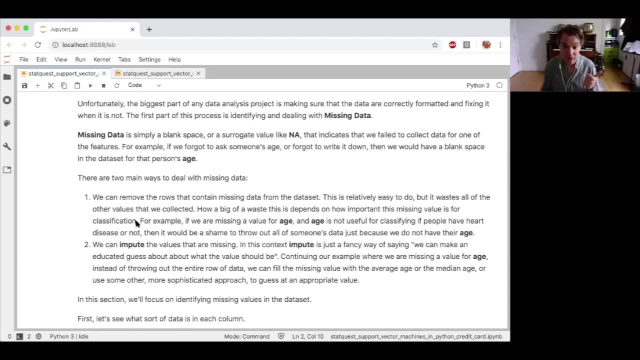 then we would have a blank space in the data set for that person's age. There are two main ways to deal with missing data. We can remove the rows that contain missing data from the data set, or we can impute the values that are missing. 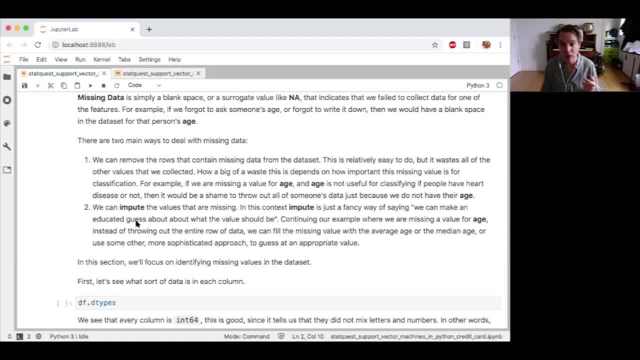 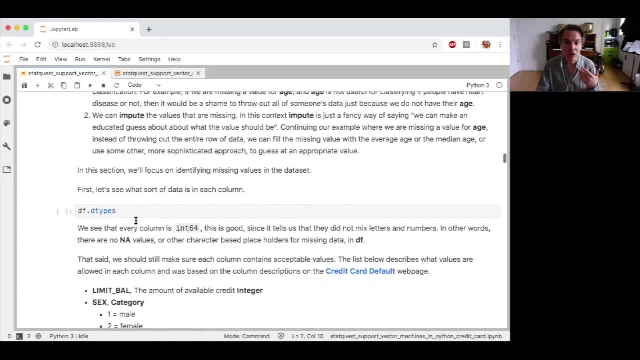 And in this context, impute is just a fancy way of saying we can make an educated guess about what that value should be. So in this section we're going to focus on identifying missing data in the data set. First let's see what sort of data is in each column. 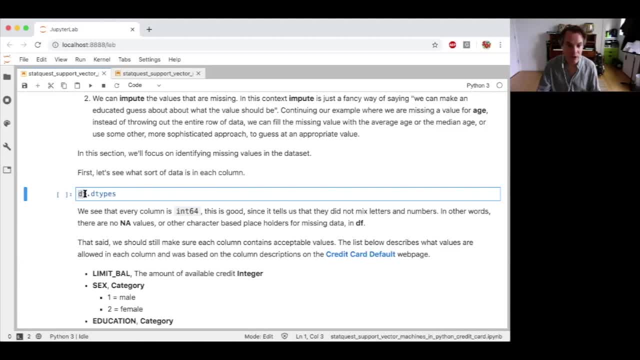 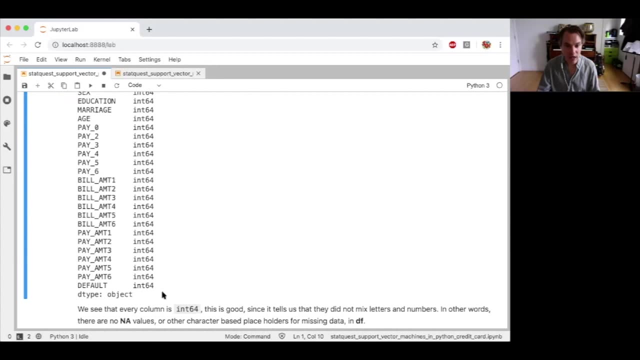 To do that. we've got our dataframe and we're asking for the data type. So we're going to check out the data types with the dtypes command And when we run that code we see that every column is int64,. 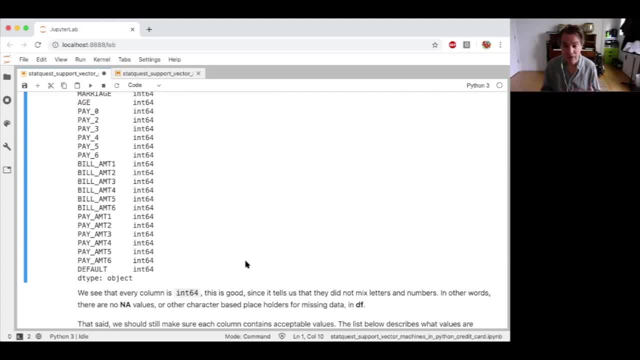 which is good, or at least it looks good- because it doesn't tell us off the bat that the person mixed letters and numbers. In other words, there are no NA values And that suggests that maybe things are in good hands because they didn't use character-based placeholders. 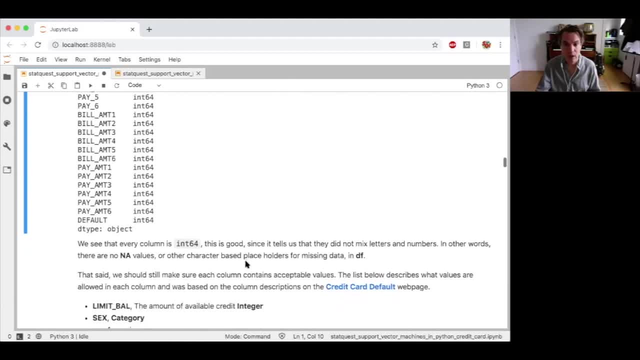 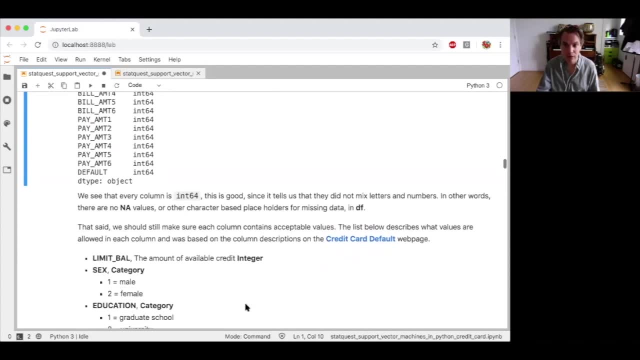 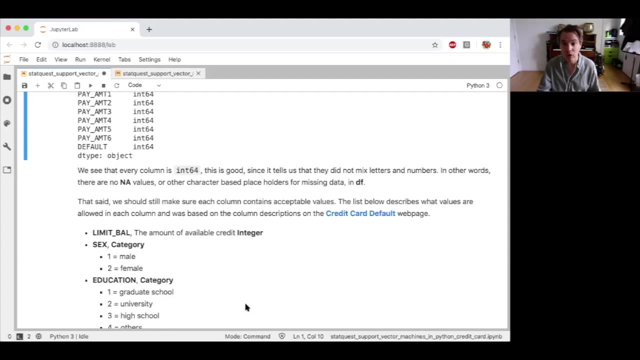 for missing data in dataframe. That said, we should still make sure that each column contains acceptable values. The list below describes what are allowed in each column and it was based on the column descriptions on the credit card default web page. So the limit balance, so the credit balance. 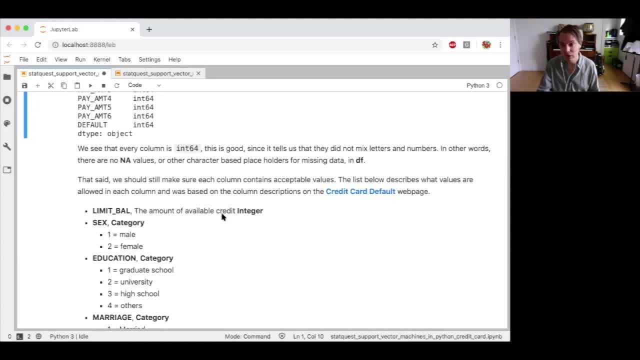 or credit limit, excuse me, is the amount of available credit and that's an integer. Sex is a category. We have one for male and two for female. Education is also a category. We've got four categories for that. Graduate school is one. 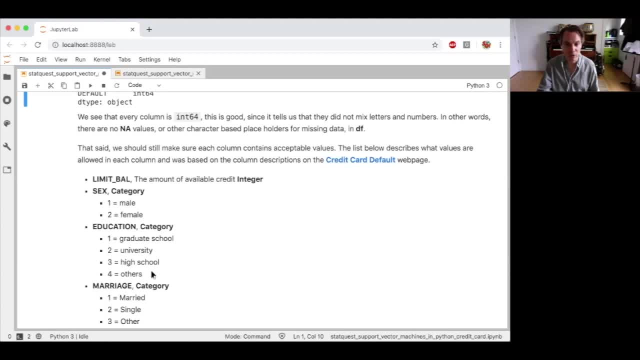 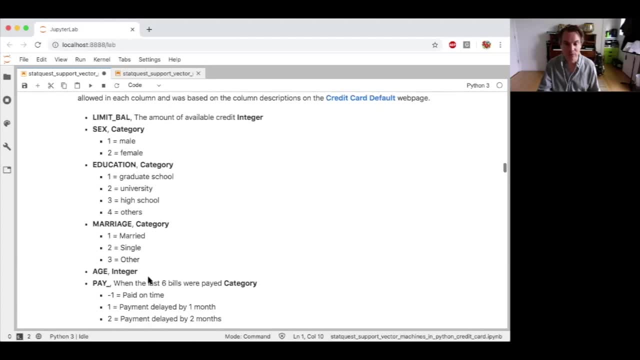 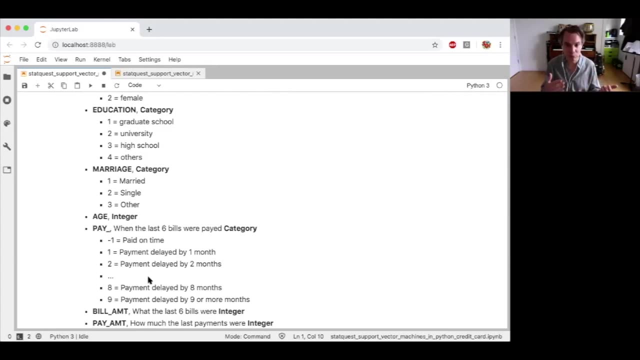 Two equals university, Three is high school and four is others. Marriage is also a category. We have one for married, two for single and three for other. Age is an integer Pay. These are a series of columns that tell us when the last six bills were paid. 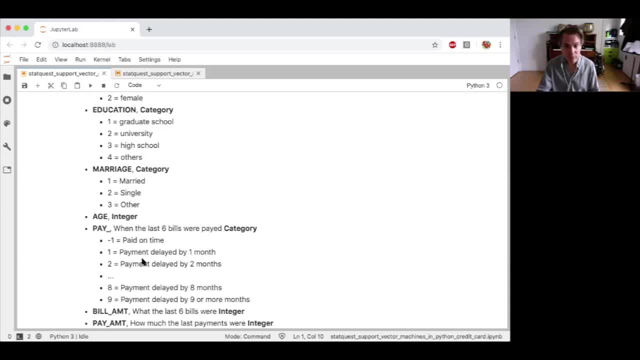 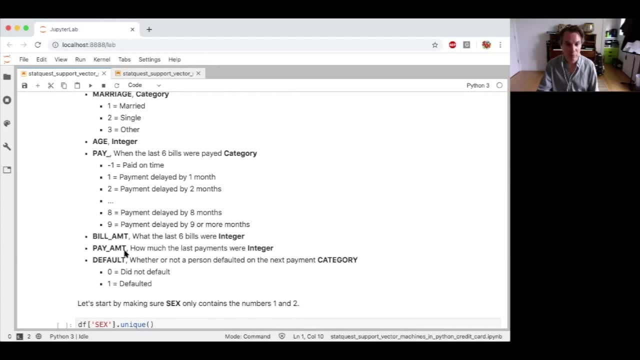 Negative one means on time, And then we have how much after that we've got, how much it's been delayed. We've got bill amount, pay amount and default, which is a binary column that has zero for did not default and one for defaulted. 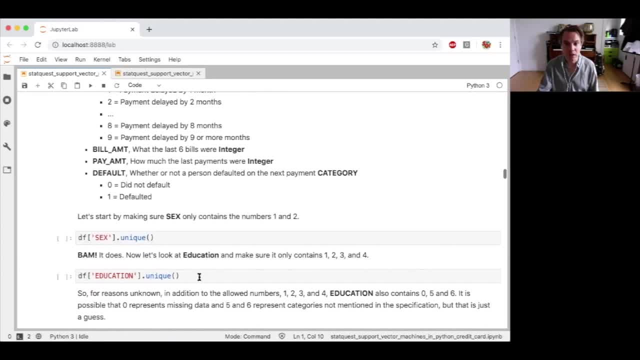 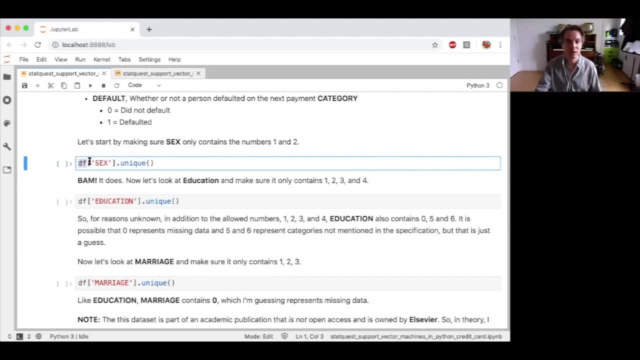 So we're going to start by making sure sex only contains numbers one and two, And we do that with our data frame And in square brackets we specify that we want to look at the column named sex And we've got that in single quotes. 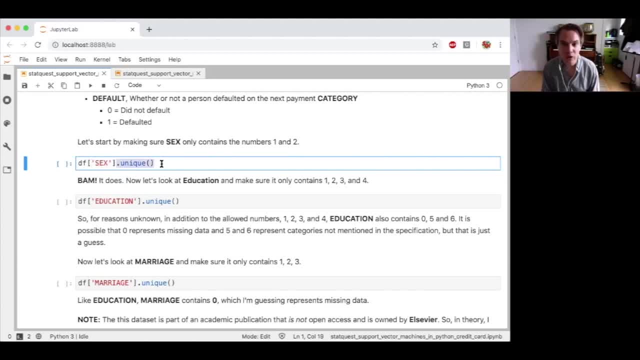 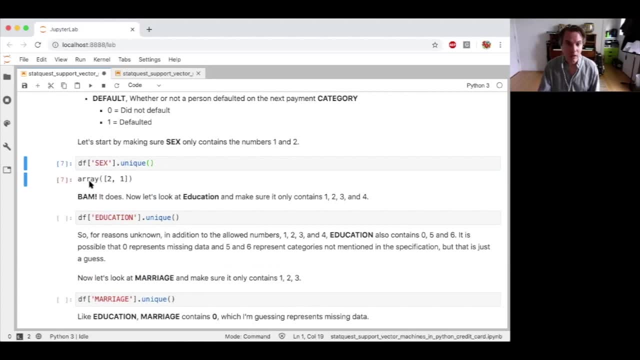 And what we want to do is we want to look at the unique values in that column And we do that with the unique function, So let's run that And we see that the unique values in this column named sex are two and one. 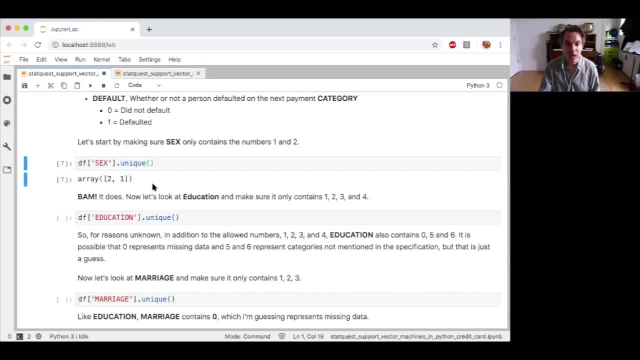 So bam it does. Now we're going to look at education to make sure it only contains one, two, three and four. So we do the exact same thing we did before, only we swapped sex with education. When we run that. 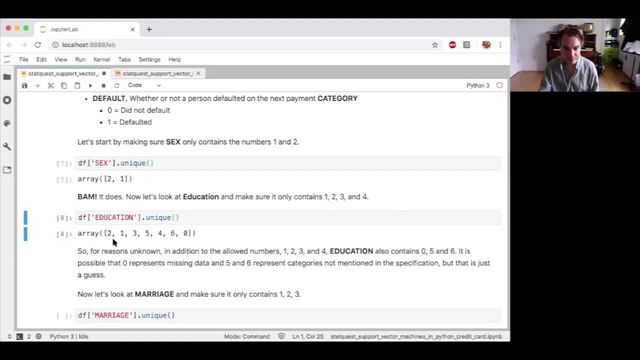 we see that, for reasons unknown, in addition to the allowed numbers one, two, three and four, education also contains zero, five and six. It is possible that zero represents missing data And five and six represent categories not mentioned in the original specification. 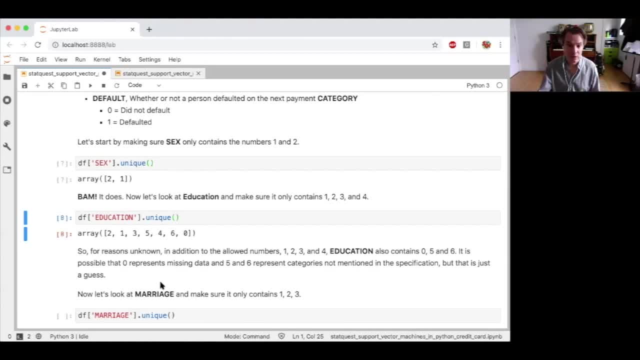 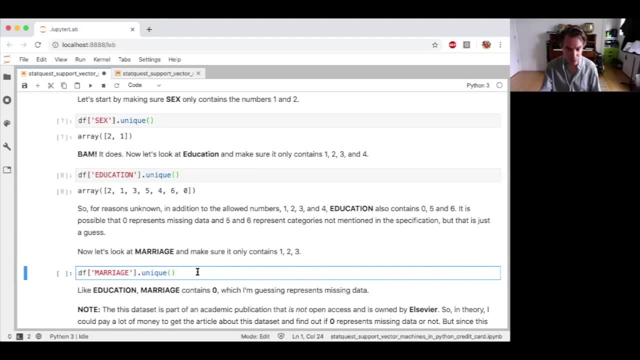 But that's just a guess. Now we're going to look at marriage and make sure it only contains one, two and three. So we do that: The exact same code as before, only this time we're specifying the column named marriage. 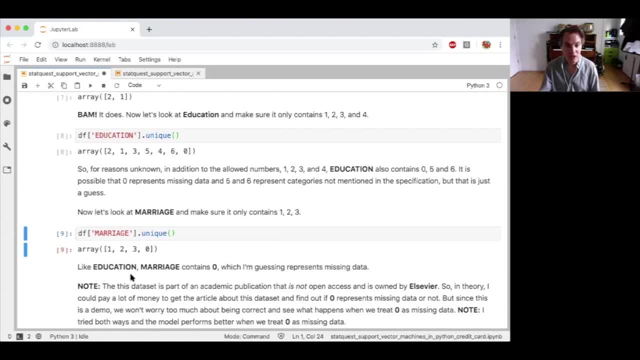 And, like education, marriage contains zero, which I'm guessing represents missing data. Now note: this data set is part of an academic publication that is not open access. It's owned by a company called Elsevier, So in theory, I could pay Elsevier a lot of money to get the article. 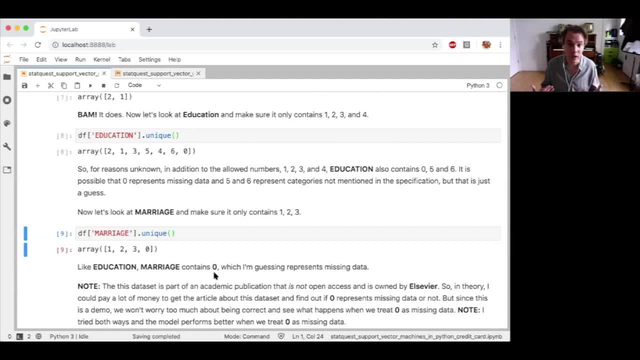 and find out if zero represents missing data or not. There's a good chance that the authors didn't even mention it in the article. So there's a good chance that even if I paid a lot of money for the article, I still wouldn't know. 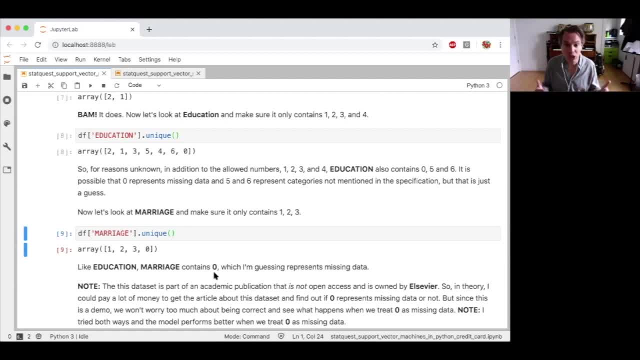 And because this is just a demo, I'm not going to worry too much about being correct And instead we're just going to see what happens when we treat zero as missing data. And I will give you, I will say this: I tried it both ways. 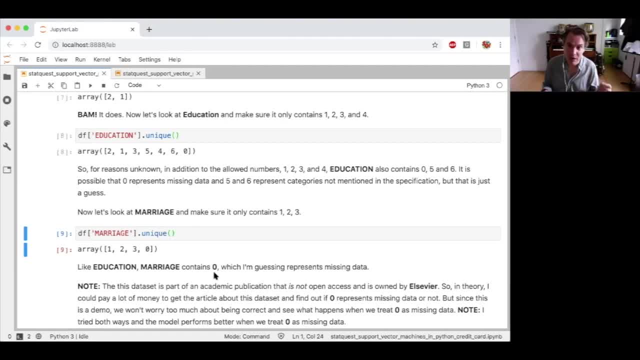 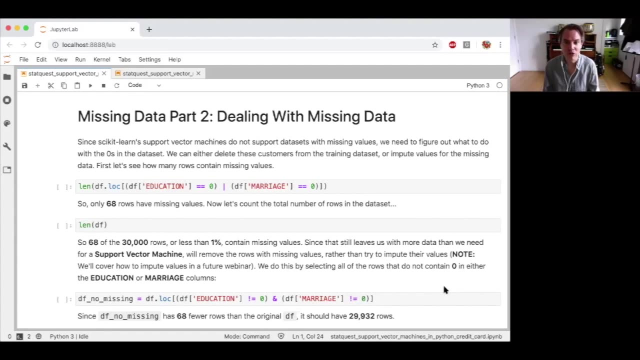 And the support vector classifier performs better when we treat zero as missing data. So I at least tried it both ways And I said, well, since it works better this way, we'll just assume that that means missing data, Since scikit-learn support vector machines do not support data. 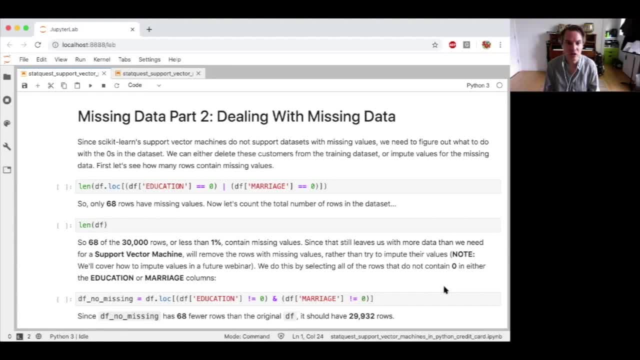 we need to figure out what to do with the zeros in the data set. We can either delete these columns from the training data set or impute values for the missing data. First, let's see how many rows contain missing values. We do that by using the loc or location function. 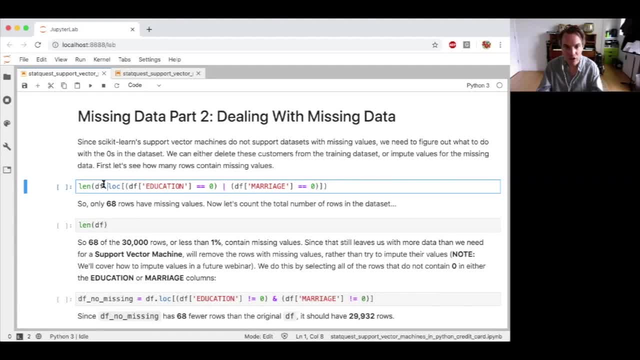 that is associated with our data frame, And what you do is you specify the number of rows and you specify sort of a logical statement that, if it's true, it'll return those specific rows that we're interested in. And what we're interested in is we're interested in finding rows. 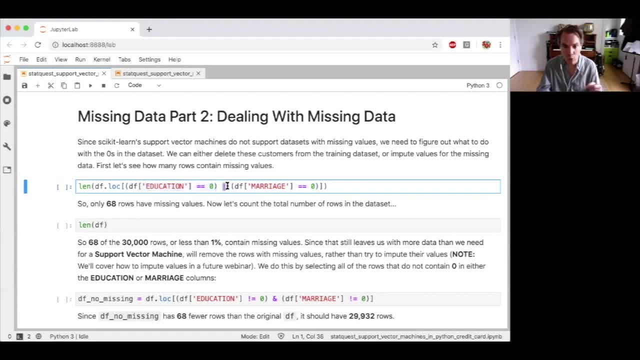 that have zero in the education column, or, and that's a logical or, and in old school computer language talk we call that a pipe, The pipe character, but it's a logical or. So we want all the lines in the data set. 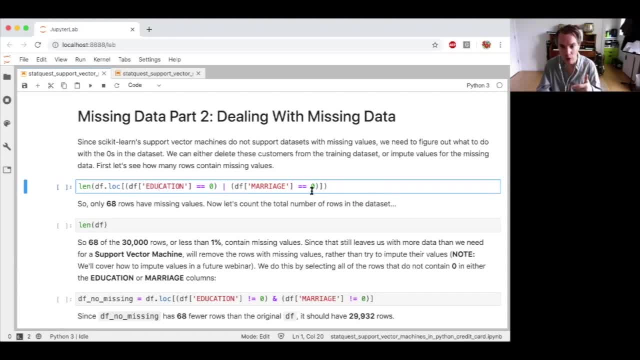 where there's a zero in the education column or there's a zero in the marriage column, And we wrapped all of this up in the lin function, which is short for length, And so we're going to count the number of rows that have zeros in those columns. 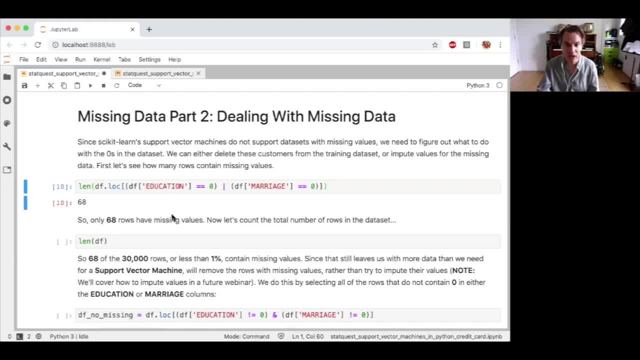 And when we run that we see that there are 68 rows that have missing values. So now we're going to count the total number of rows in the data set And we're going to use that lin or length function, just like we did before. 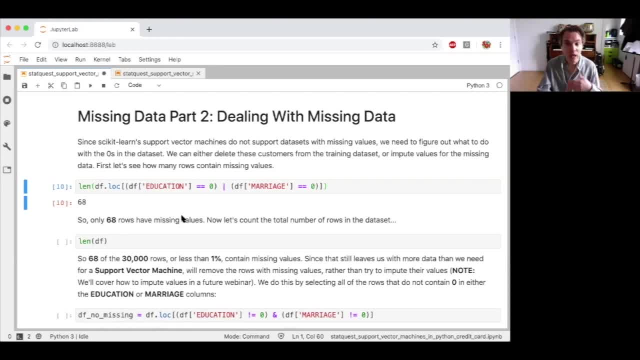 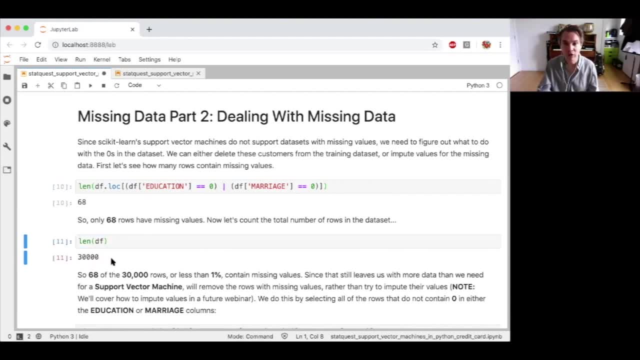 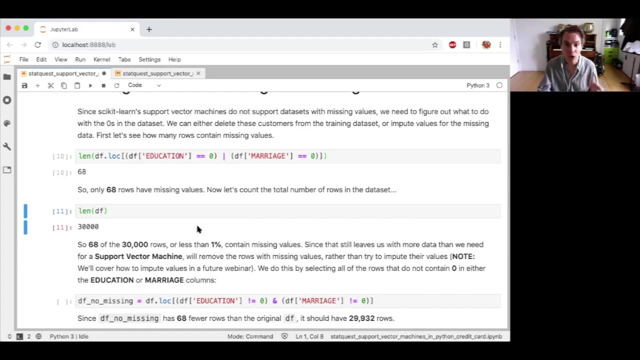 only this time we're not specifying which rows we want, And when we don't specify specific rows, we get them all And we see that there are 30,000 rows in the data set to begin with, And so 68 of the 30,000 rows or less than 1%. 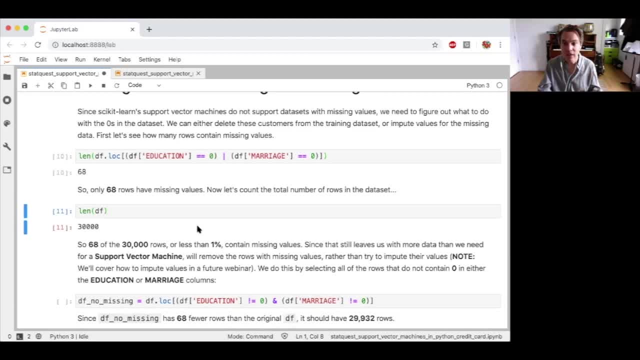 contain missing values. Since that still leaves us with more data than we need for a support vector machine, we will remove the rows with missing values rather than try to impute their values And, like I said, we're going to try to do imputing imputation. 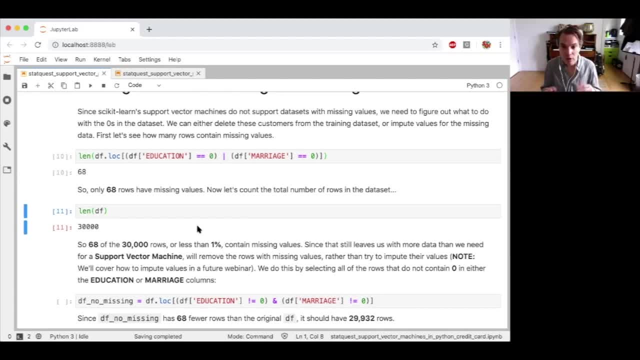 in a future webinar, hopefully in two months. So the way we do this, we select all the rows that do not contain zero in either education or marriage, And the way I said that was a little awkward, because we're actually going to use an and 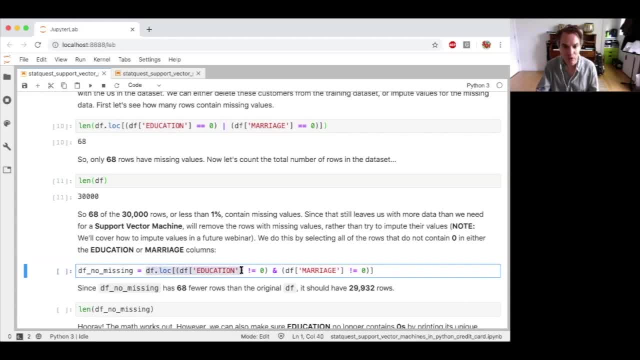 a logical and in this statement. So, just like before, we're getting all the rows. We're using this loc function to get the rows where this logical statement is true, And what we want are rows that do not have zero in education and do not have zero in marriage. 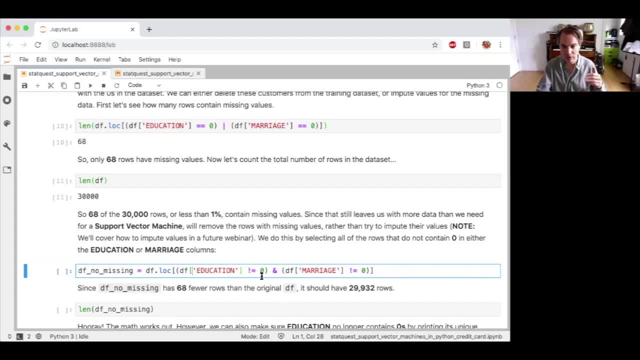 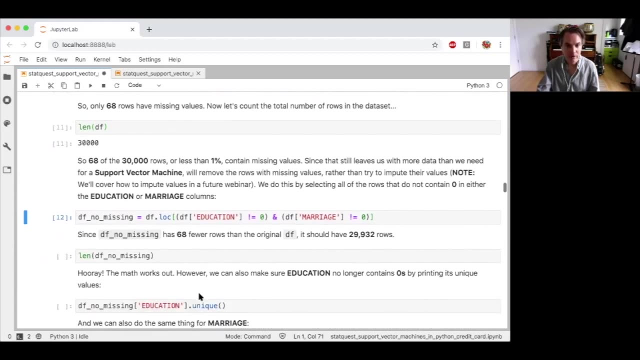 And we're going to save all those rows that don't have zeros in education and they don't have zeros in marriage. We're going to save all those rows in a new data frame called data frame no missing. So we'll run that. And since data frame no missing. 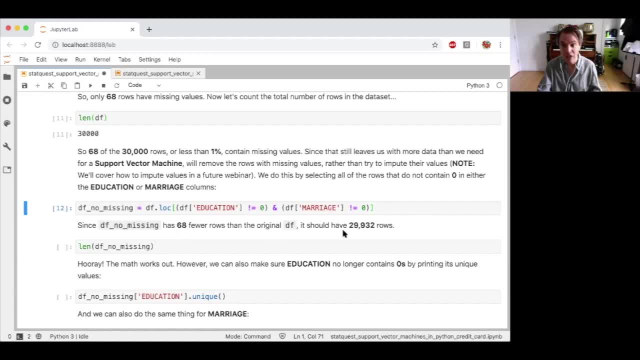 has 68 fewer rows than the original data frame. it should only have 29,932 rows, So we're going to count the number of rows using that length function again. And there we got it. Hooray, the math works out. 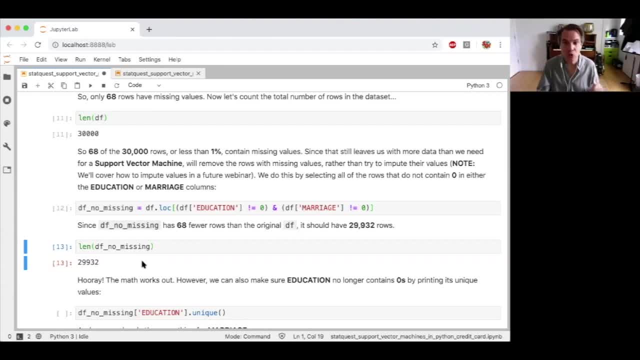 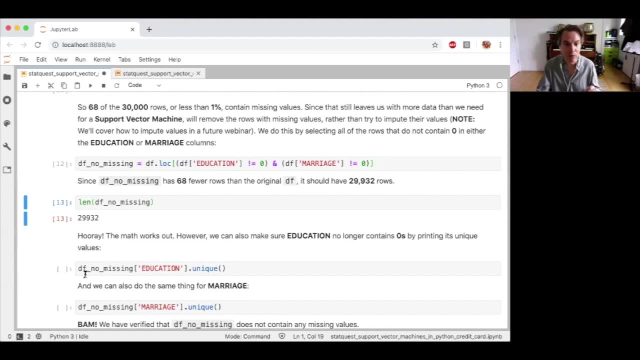 However, we can also make sure that education no longer contains zeros by printing out the unique values. This is exactly what we did before. However, now we're specifying data frame- no missing- rather than just data frame- the original data set- And now we see that there's no zero there. 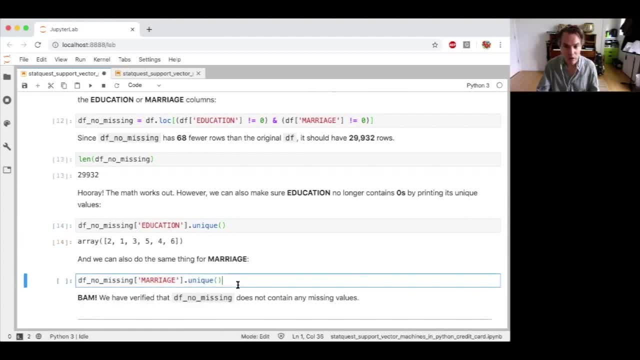 And when we do the same thing for marriage, we print out the unique values for marriage. Now we just have one, two and three. So bam, We have verified that data frame. no missing does not contain any missing values. All right. 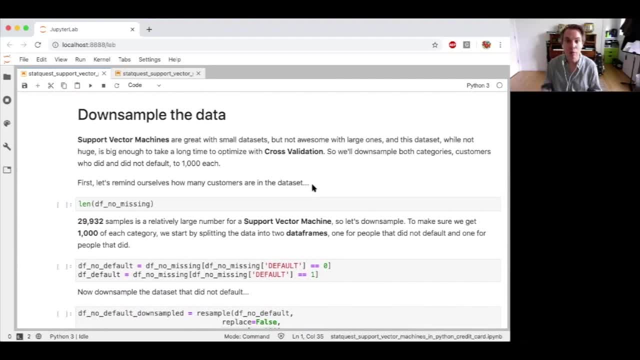 And we're ready to move on to the next section, where we downsample the data set. So, like I've said, support vector machines are great with small data sets. The data set that we used for classification trees is relatively small and support vector machines do pretty well. 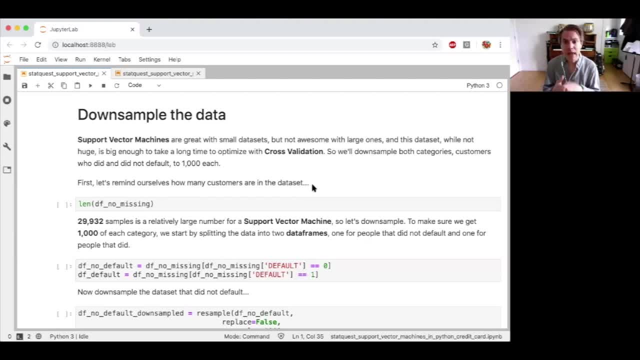 with that data set. However, like I said, they can take a long time with large data sets, and this is relatively large. So we're going to downsample both categories: customers who did not default and customers that did down to 1,000 each. 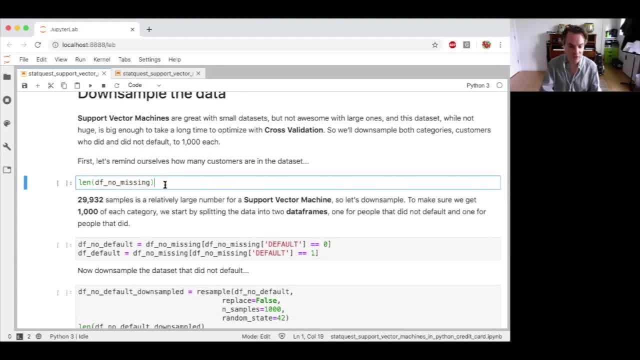 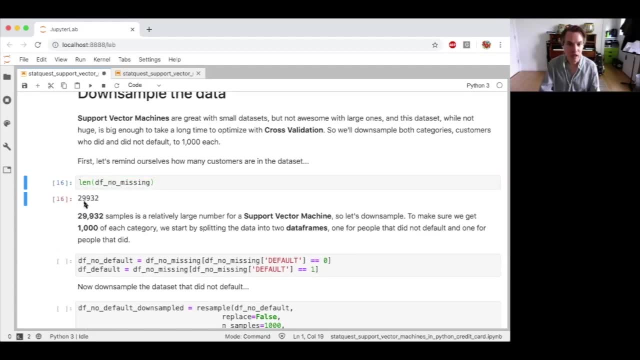 So first thing we're going to do is just remind ourselves how many rows of data we're working with, because we removed some of them. So we use the length function again and that tells us we've got 29,932 samples. That's relatively large. 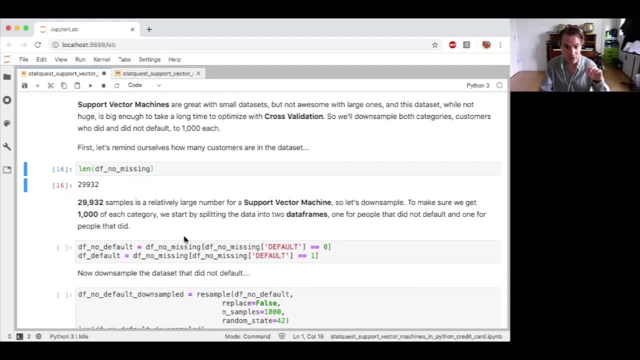 so we're going to downsample it to 1,000 of each category. So the way we do that is: we've created this, we've already have this data frame called data frame new- missing, and we're specifying we want all the rows. 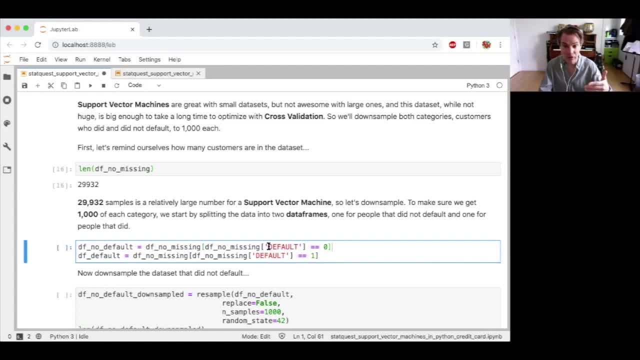 where someone did not default. so default is zero and we're going to store that in a new variable called df- no default. And then we're doing the same thing for the people that defaulted. We're storing them in another data frame, So we're splitting the data. 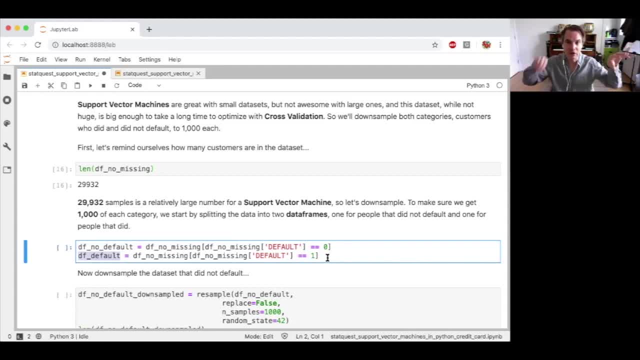 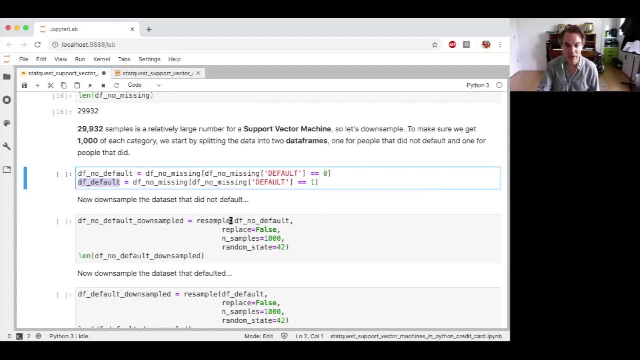 into two variables here: one for people that defaulted and one for people that did not default. And now what we're doing is we're downsampling the people that did not default. We're using the resample function and we're passing it- the data frame. 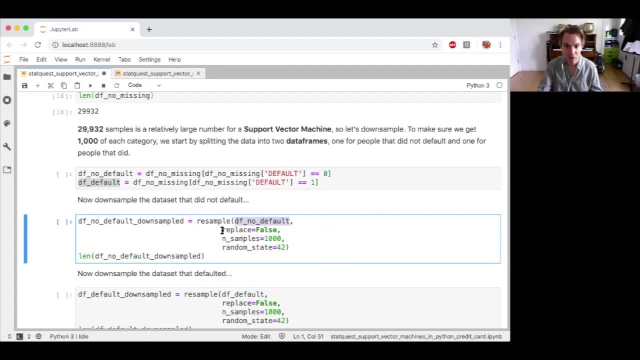 that consists of people that did not default. We're setting replace to false, so that means when we pull something out of there, we don't and we put it in our new data frame. we don't put that back in the pool of possible people that we could select again. 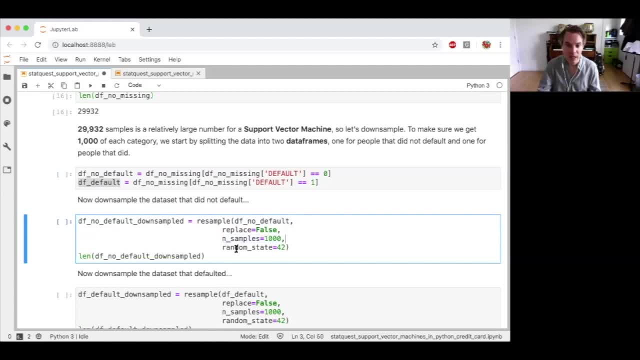 And we're saying that we want 1,000 samples and we're setting the random state to 42. That's a random seed, and all that does is make sure that you get the same answer that I get, And then what we're going to do. 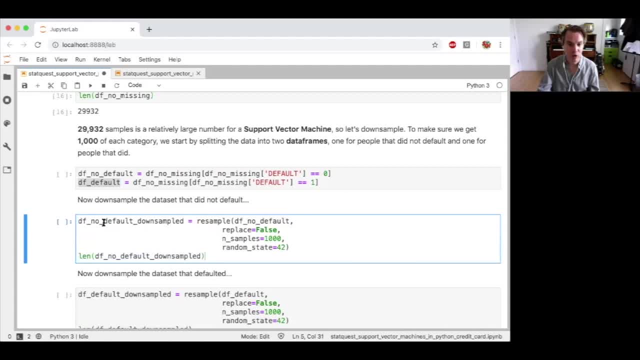 is we're going to print out the length of this new data frame that we're creating. data frame: no default downsampled, So let's run that. Oh no, I got there too early. I didn't split the data set into half. 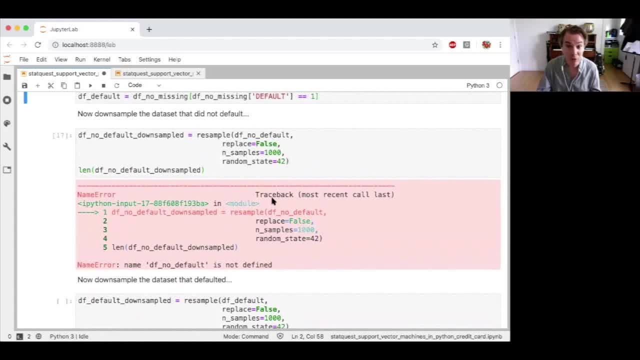 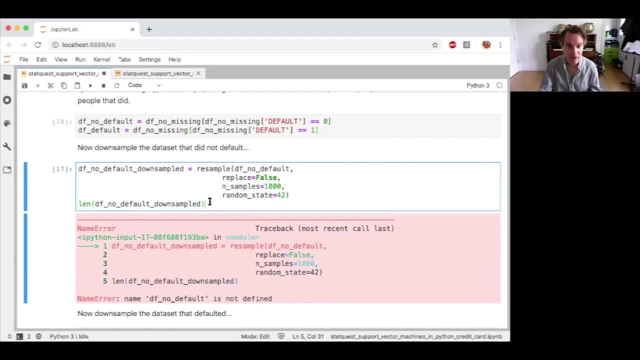 So yeah. So when you see this pink, that means something went wrong, And instead of feeling great shame, what you got to do is just got to debug it. And so let's rerun this again, because the first time I ran it 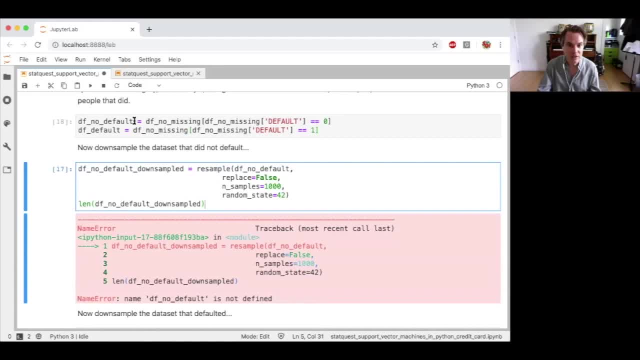 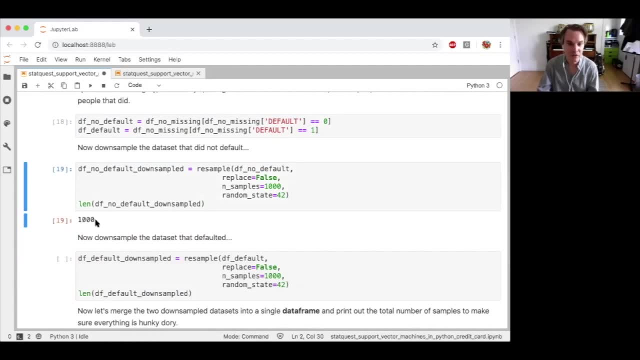 I hadn't run this chunk of code first, And so this data frame no default. this guy did not exist, But now it exists. So let's see what happens, And it runs and tells us we've got 1,000 rows in our new data frame. 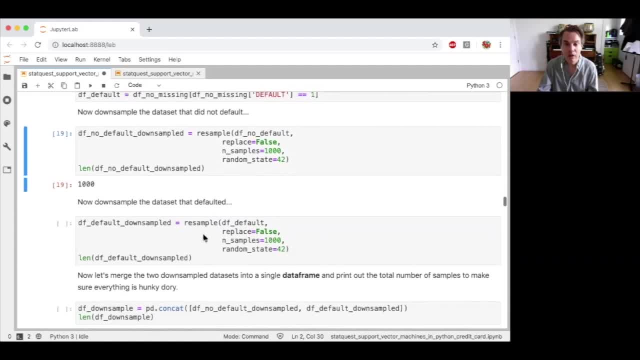 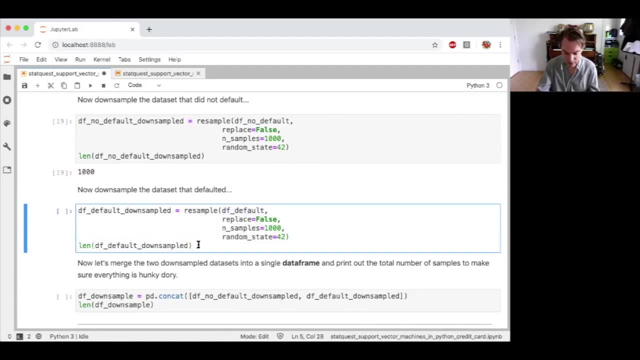 data frame: no default downsampled. Now we're going to do the exact same thing, but this time we're using the people that defaulted And we're going to print out the number of rows there and there. So we've got two new variables. 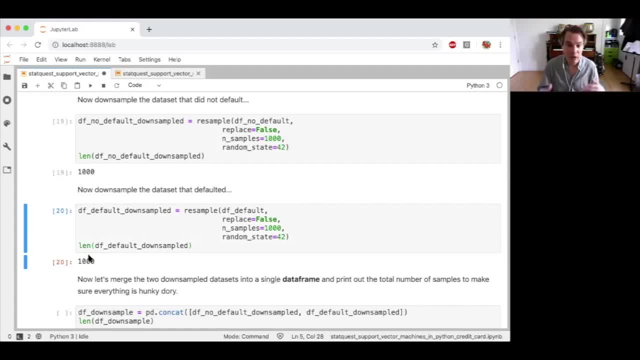 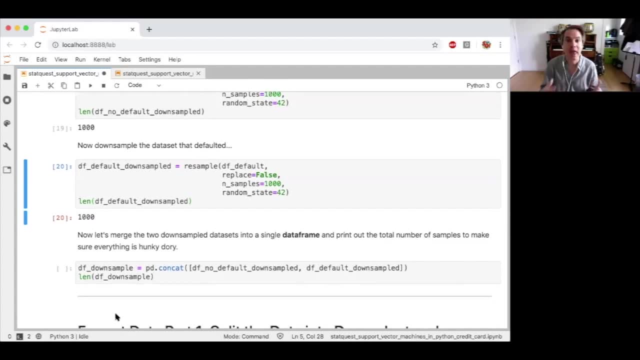 each containing 1,000 rows each. And now what we want to do is we want to merge them back into a single data frame and print out the total number of rows, to make sure everything is hunky-dory. To merge the two data frames that we're creating. 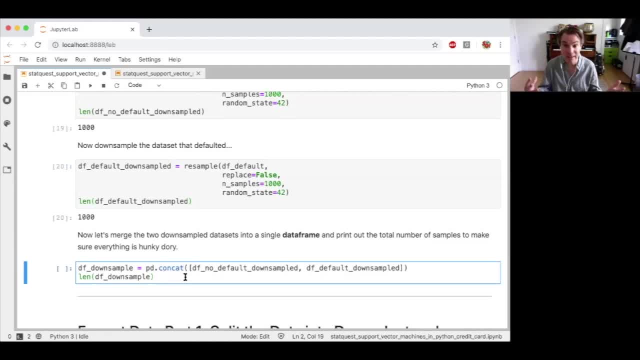 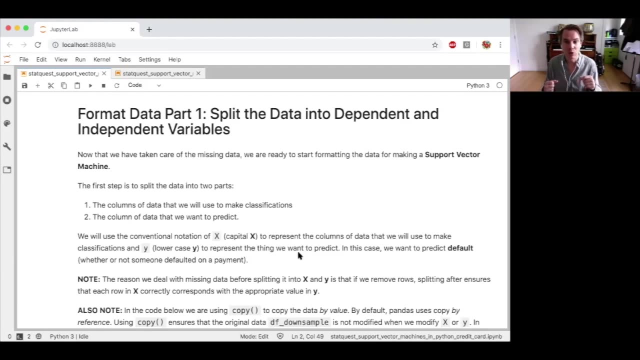 we're using this pandas function called concat, which will concatenate the two things. So there we go, Bam 2,000.. So now that we've taken care of the missing data, we are ready to start formatting the data for making a support vector machine. 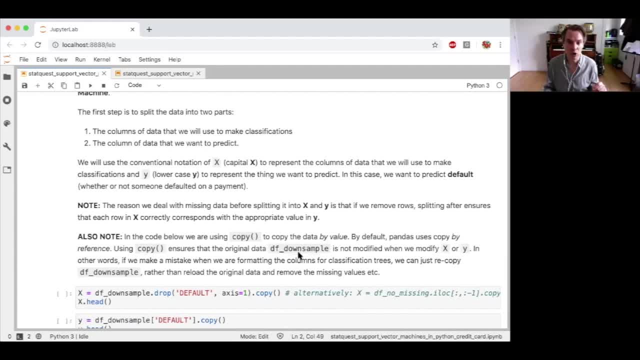 The first step is to split the data into two parts. We're going to have one part that contains the columns of data that we will use to make classifications, and one part is going to be a column of data that contains the things we want to predict. 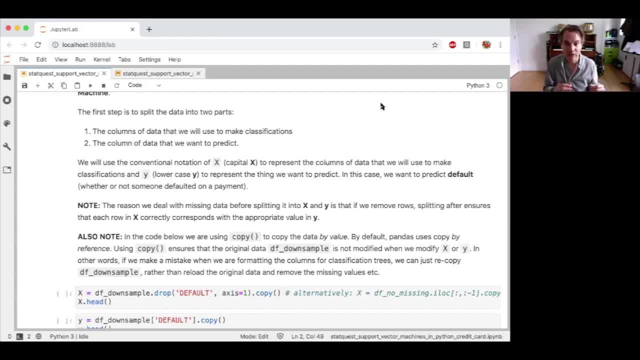 So we're going to use the conventional notation of capital X to represent the columns of data that we will use to make classifications, and we're going to use lowercase y to represent the thing we want to predict. In this case, we want to predict default. 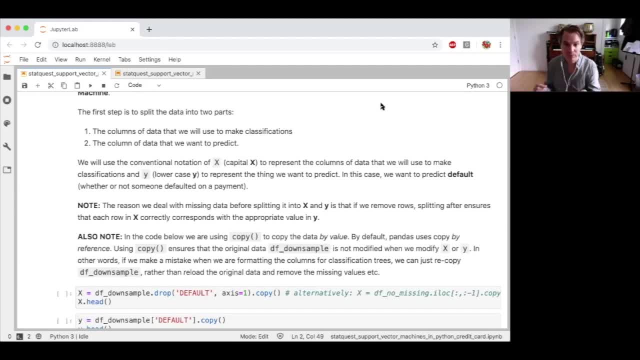 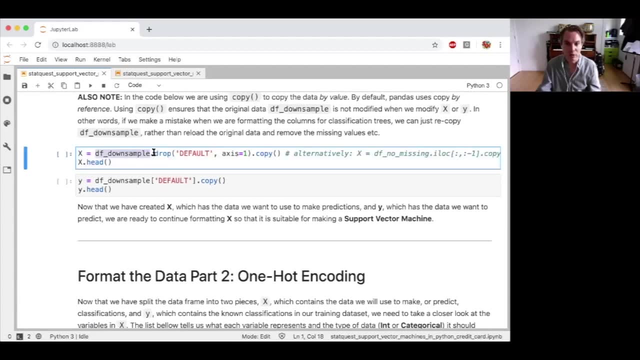 whether or not someone defaulted on their payments. So here's how we're going to do that. We've got our downsampled data set and what we're doing is we're going to drop the default column and we're going to copy that. 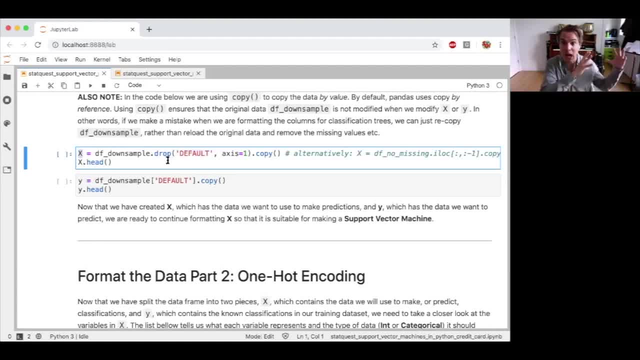 and we're going to store that into uppercase X and that's going to be our set of columns that we're going to use to make predictions, and then we're going to print out the first five rows. So let's do that, Bam. 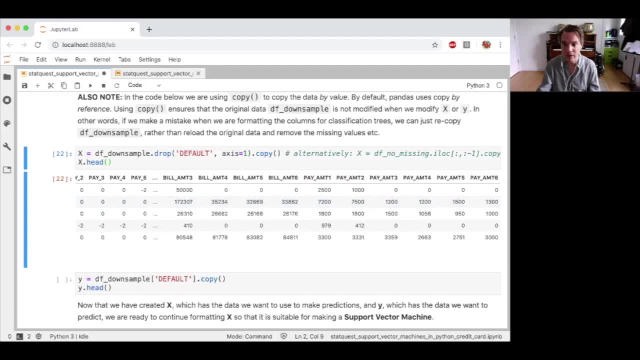 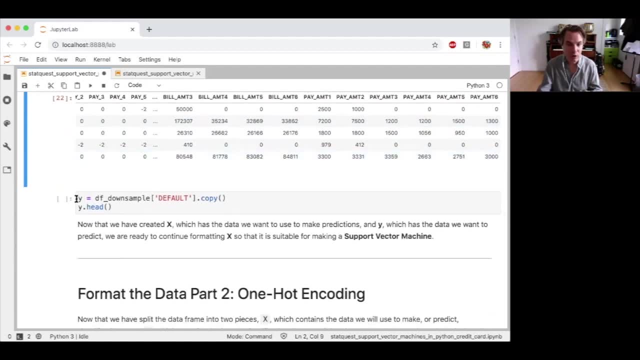 Okay, you'll notice when we scroll over to the right we no longer have that column called default, So this data set does not contain the thing we want to predict. Now, here we're going back to that data frame that contains the downsampled samples. 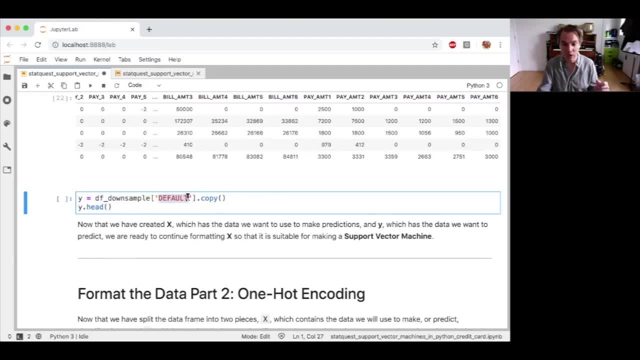 and now we're just specifying that one column default and we're making a copy of it and we're storing it in a new variable called y, and then we're going to print out the first five rows. Bam, Okay, now we've created uppercase X. 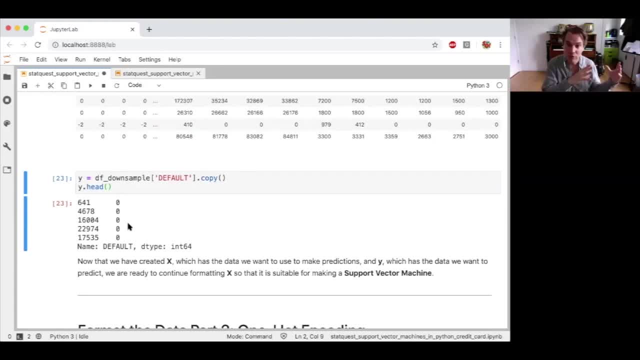 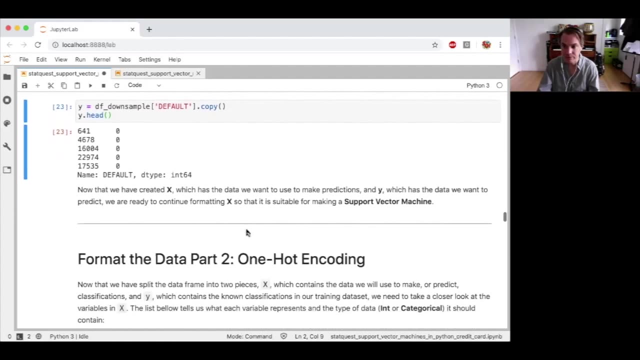 which is the data we're going to use to make predictions, and lowercase y, which has the data we want to predict. We are ready to continue formatting X over here so that it's suitable for making a support vector machine. Okay, so now we're on to one hot encoding. 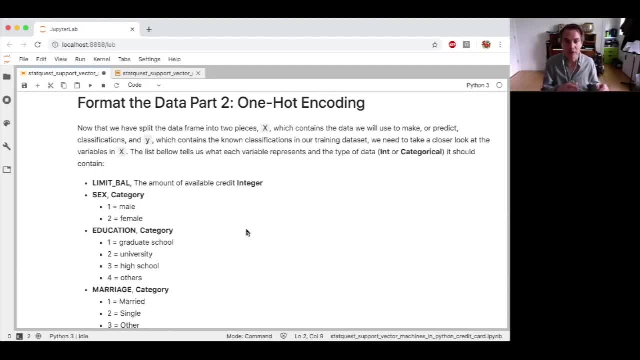 Now we have to split the data frame into two pieces. uppercase X, which contains: Okay, we've already done this, We've split things up. Now what we need to do is take a look at the variables in X, and this list tells us whether the variable is supposed to be. 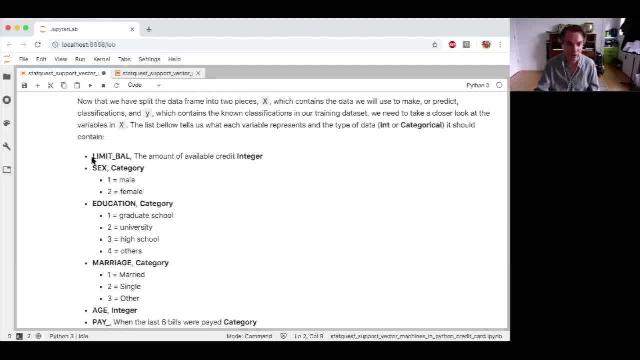 an integer or a category. So we see limit balance as an integer, That's the credit limit. Sex is a category, That's male, or one for male, two for female. Education has a bunch of categories: one, two, three and four. 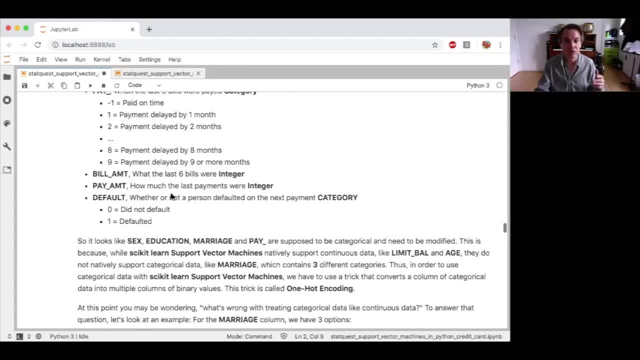 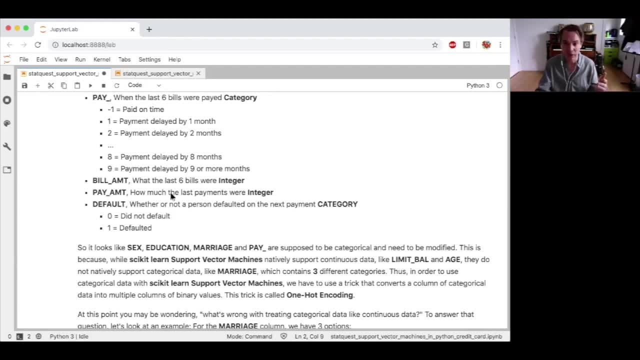 We've already talked about these. Okay, so it looks like sex education, marriage and pay are supposed to be categorical And they need to be modified. This is because scikit-learn support vector machines, while they natively support continuous data. 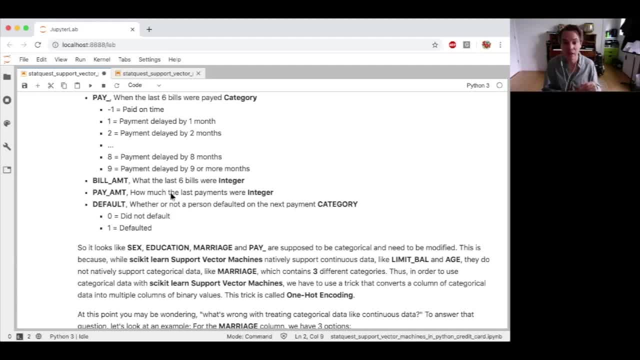 like limit, balance and age. they do not natively support categorical data like marriage, which contains three different categories. Thus, in order to use the categorical data with scikit-learn support vector machines, we have to use a trick that converts the column of categories. 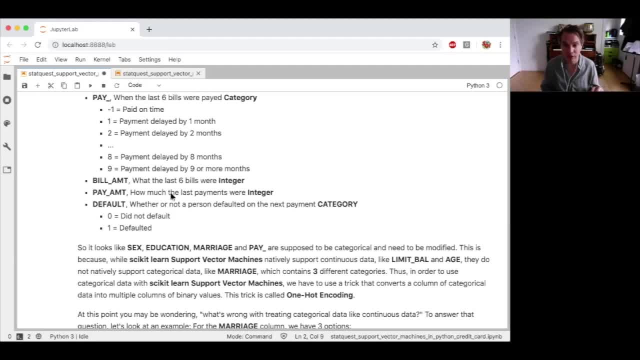 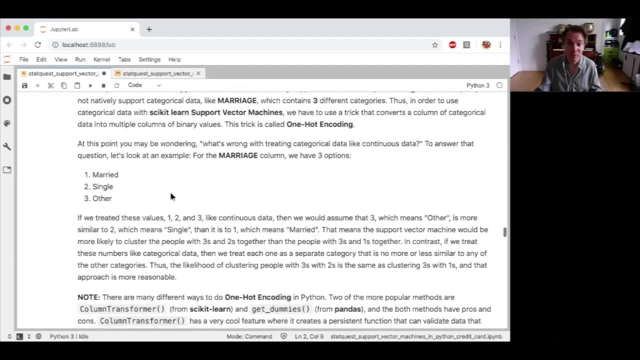 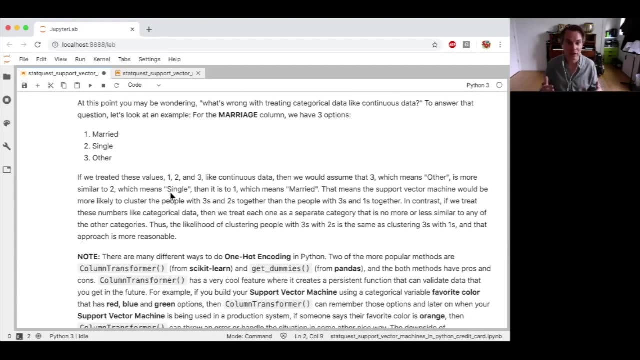 into multiple columns of binary values, And this trick is called one-hot encoding. So at this point you may be wondering what's wrong with treating categorical data like it's continuous. So to answer that question, let's look at an example. 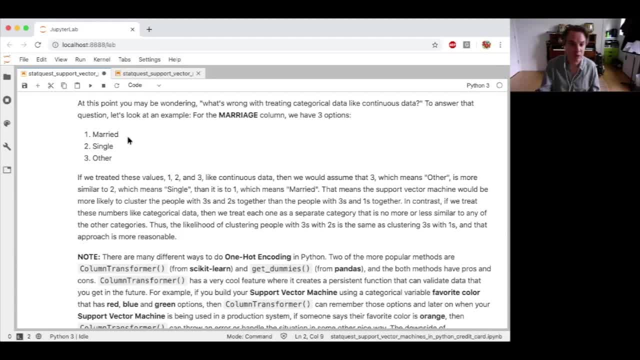 For the marriage columns we have three options: one married, two single and three other. If we treated those values- one, two and three- like continuous data, then we would assume that three, which means other, is more similar to two, which means single. 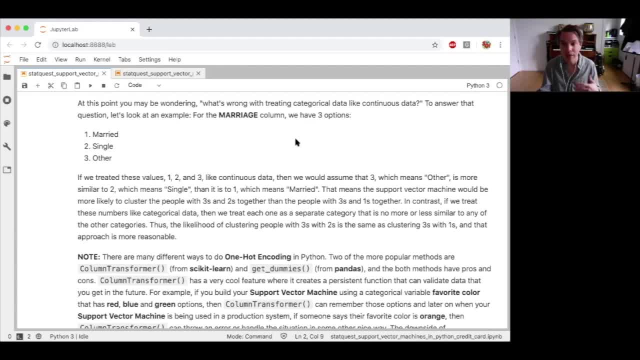 than it is to one, which means married, And that means the support vector machine would be more likely to cluster people with threes and twos together than people with threes and ones together. And, in contrast, if we treat these numbers like categorical data, then we will treat each one. 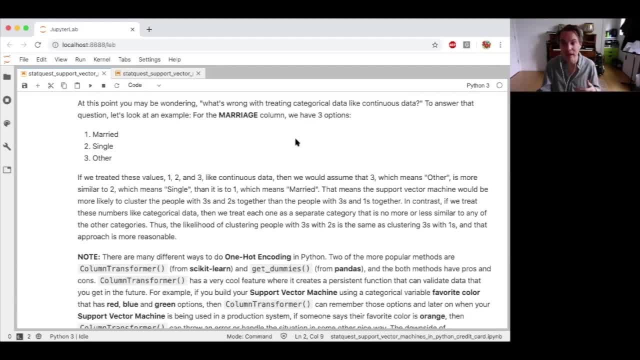 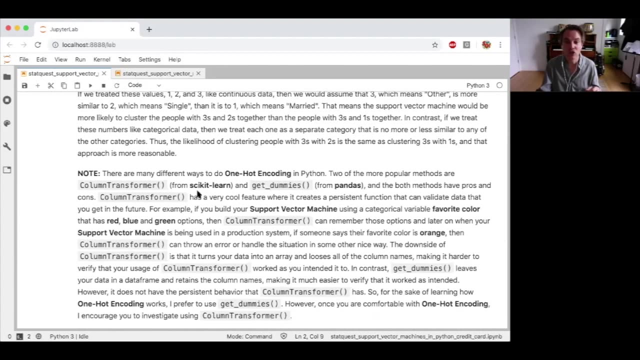 as a separate category that is no more or less similar to any of the other categories. Thus, the likelihood of clustering people with twos and threes is the same as clustering threes and ones, and that approach is more reasonable. Note: I have a huge treatise on different ways. 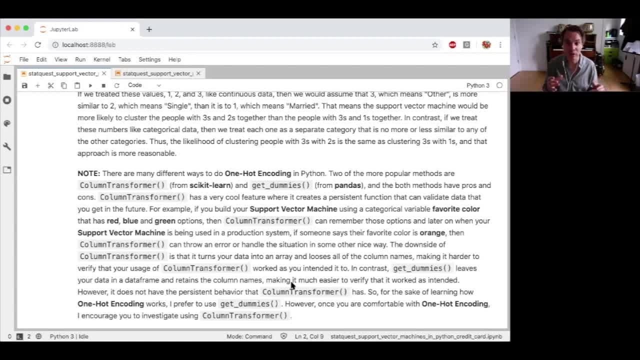 to do one-hot encoding. There's two very common ways to do it. There's a function called column transformer from scikit-learn and there's a function called get dummies from pandas, because I believe that get dummies is better for teaching how one-hot encoding. 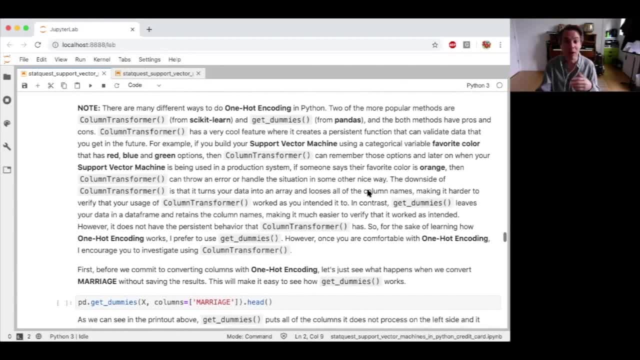 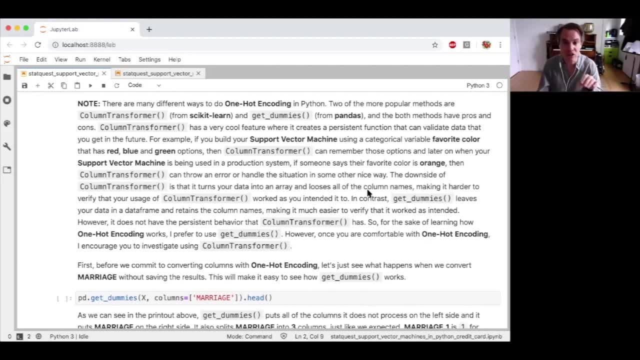 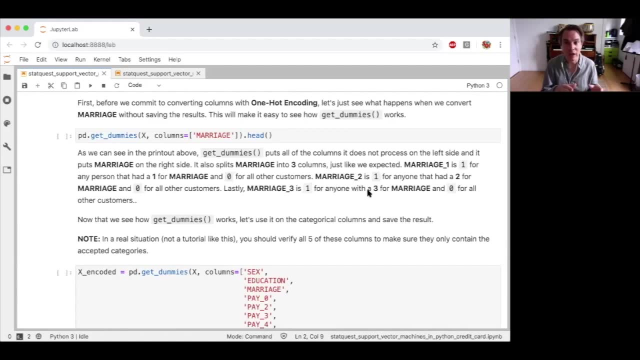 works. we're going to use it. However, just know there's alternatives, and you should definitely read this description at your leisure to learn about the pros and cons of these two different approaches. Okay, first, before we commit to converting columns with one-hot encoding, I just want to show you. 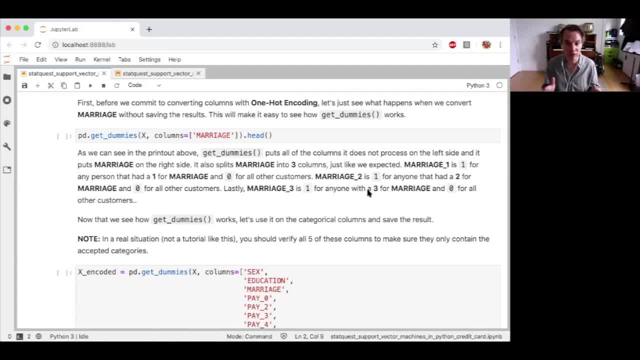 what happens when we convert marriage without saving the results. So to make this easy to see, we're going to use get dummies. Get dummies is a panda function, and so we pass it. X capital X, that's the columns that we want to transform. 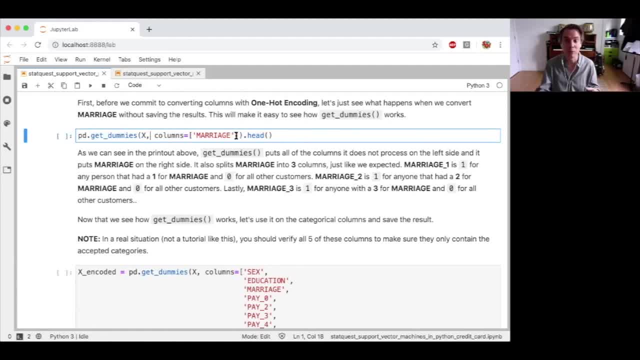 and we specify the columns that we want to transform For this demonstration. we're just going to transform marriage and then we're going to print out the first five rows to see what it did. Okay, Scroll over here and you'll see that on the left side. 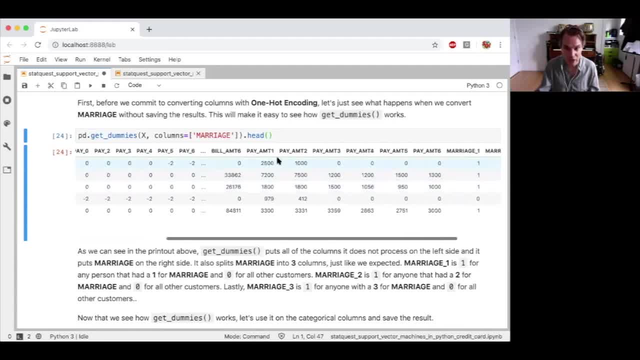 of the data frame are the columns that we did not touch, and on the right side are the columns that we did not touch, and on the right side we've got three columns for marriage. We used to just have one that contained three values. 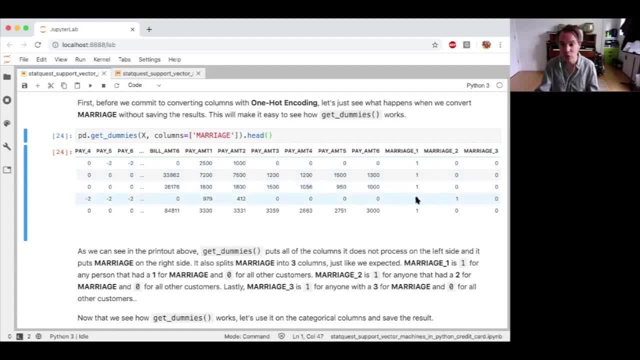 Now we have three columns and each one contains a zero and a one. One in this column, marriage one, there's a one if there was a one in the original marriage column there and a zero otherwise. For marriage two, there's a zero if or there's a one. 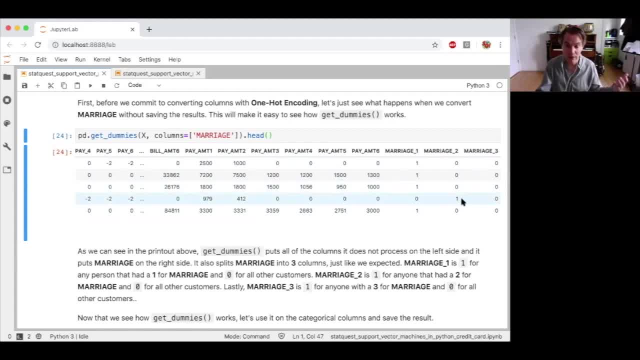 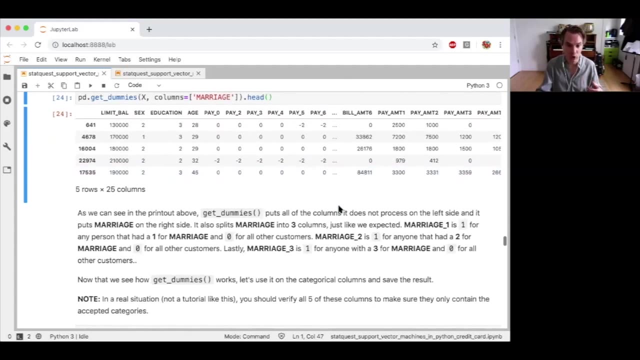 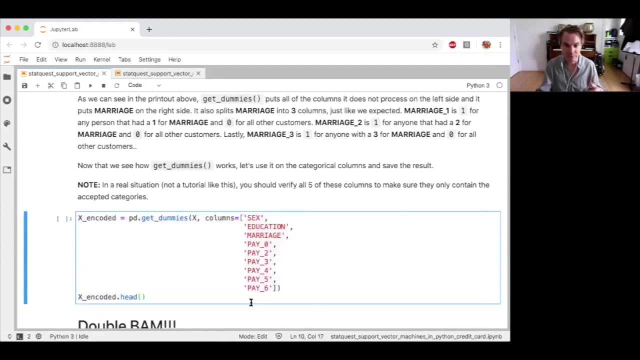 if they originally had a two in the marriage column and a zero otherwise. And marriage three is one if they originally had a three in the original column and zero otherwise. So that is how one-hot encoding works. Okay, Now we're going to do it for all of the categorical columns. 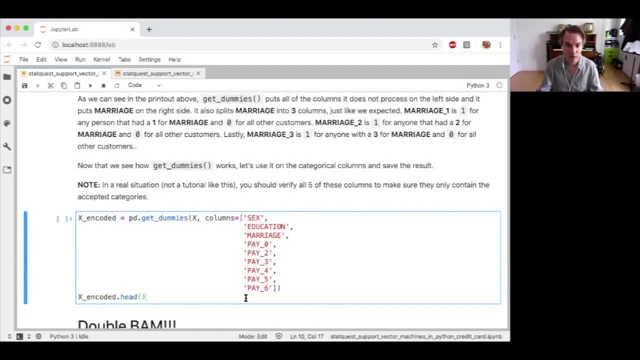 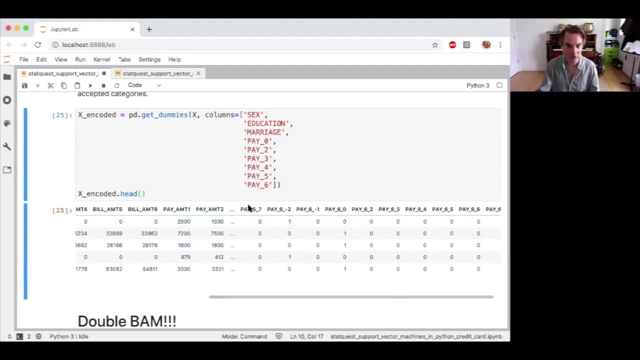 And then we're going to print out the first five rows just to see what it looks like. All right, So here is our new data frame. We've got a dot dot dot specifying that some columns are not shown. But you see that pay these columns. 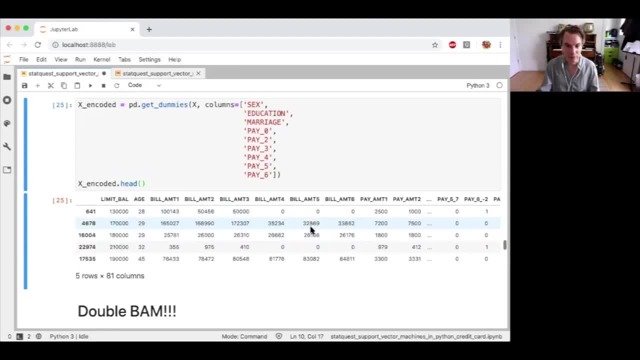 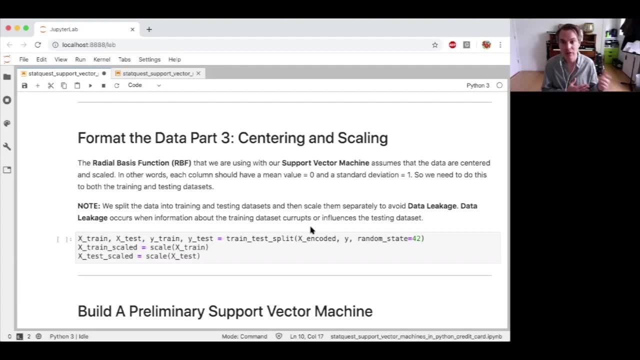 have all been converted into new columns, So double bam. The last part of formatting the data for a support vector machine is to center and scale the data. The radial basis function that we're going to use assumes that the data are centered and scaled. 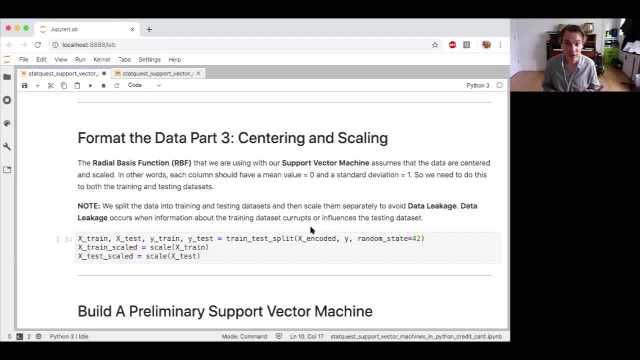 So, in other words, each column should have a mean of zero and a standard deviation of one. So what we're going to do is first: what we're going to do is we're going to split the data into training and test data sets. 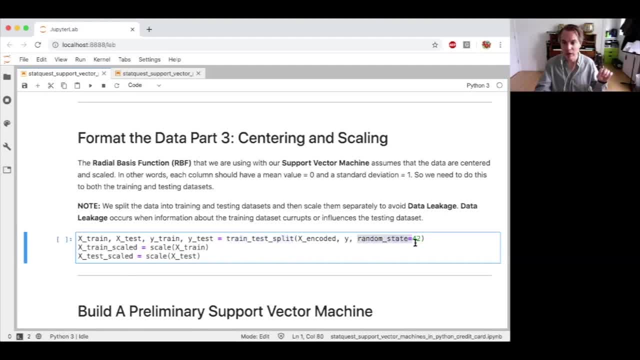 So we're using train test split Again. we're setting the random state so that you could reproduce what I've got. We're passing it in X encoded. That's the one-hot encoded X, these columns over here that are going to make the predictions. 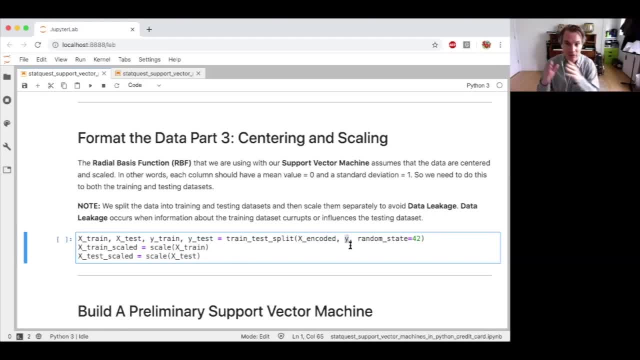 And we're passing in Y. That's the thing we want to predict And we're creating X train, X test, Y train and Y test And I believe the default setting is for 70% of the data to go into the training data set. 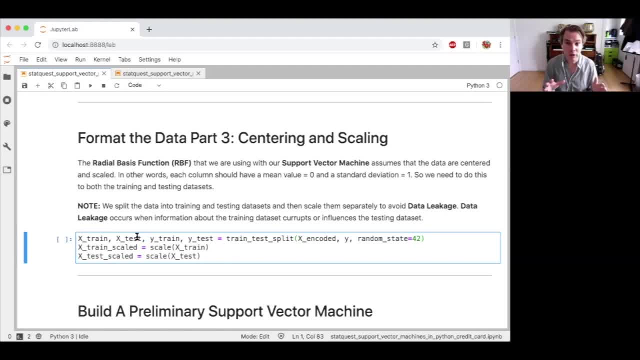 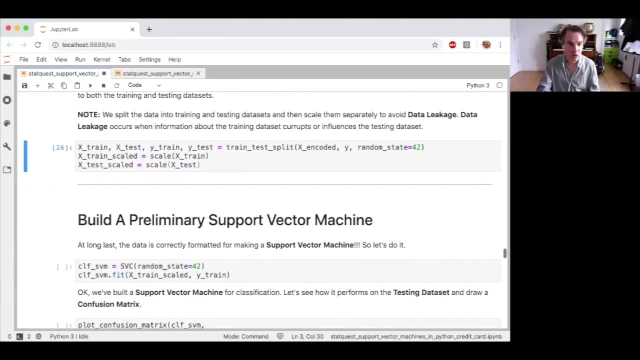 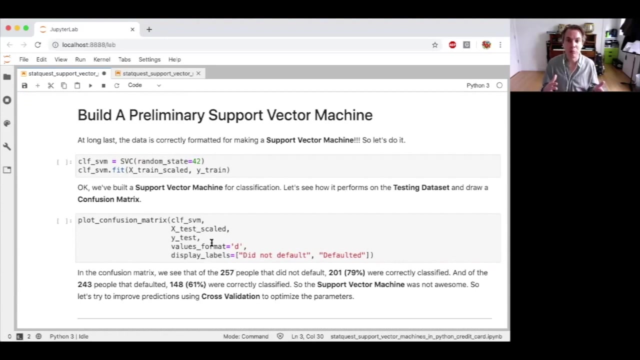 and 30% to go into testing. Don't quote me on that. I just believe that's the case. After we do that, we are scaling the data sets using the scale function, Bam. All right, Moving along. Now we're going to talk about building. 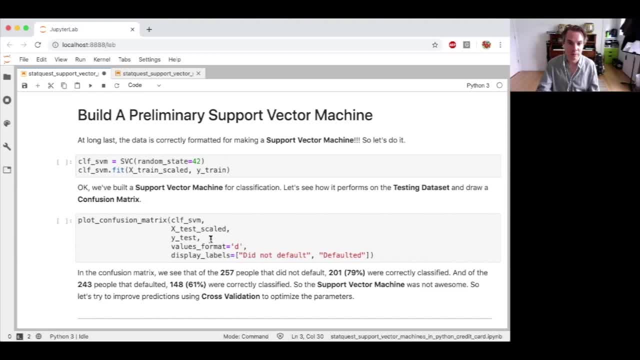 a preliminary support vector machine. We've done a lot of stuff. We've almost spent a whole hour just formatting data And now we're finally getting to the good part. The way we do that is: we call SVC for support vector classifier. We set the random state to 42.. 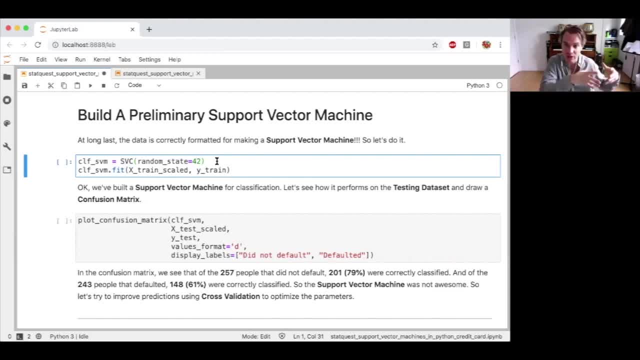 And what this does is it kind of makes an untrained shell of a support vector classifier. The next step, and we're saving that shell as classifier underscore support vector machine. The next step is to call fit using that shell. And so what we're doing is we're fitting it. 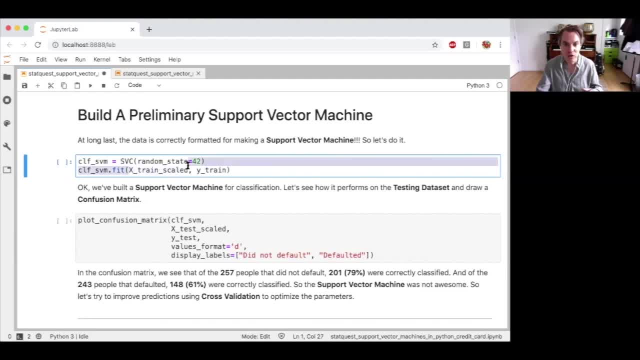 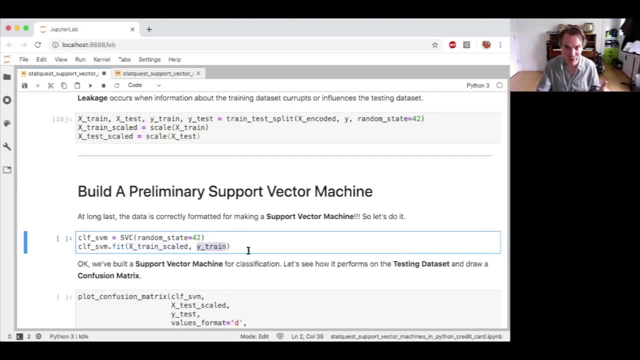 or we're training it on the training data. So we've got X train scale and Y train, And we don't scale Y train because that's just zero and one. My brain was Left, my head for a second, So anyway, so that's correct. 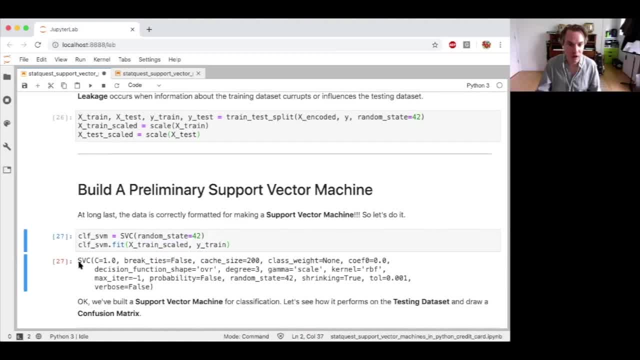 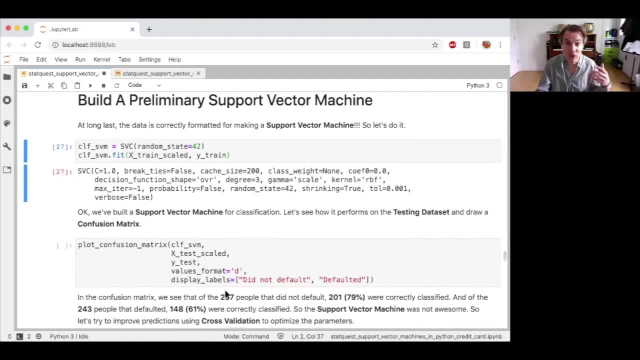 And we run it And it just prints out the support vector classifier plus the default settings that it has. And now that we've trained the classifier, we can see how it performs with a confusion matrix And we're going to use the test data set we're passing in. 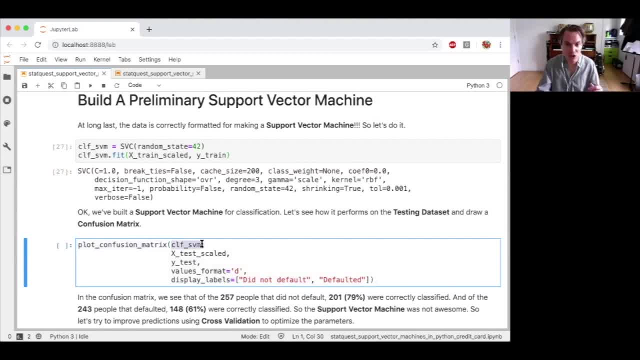 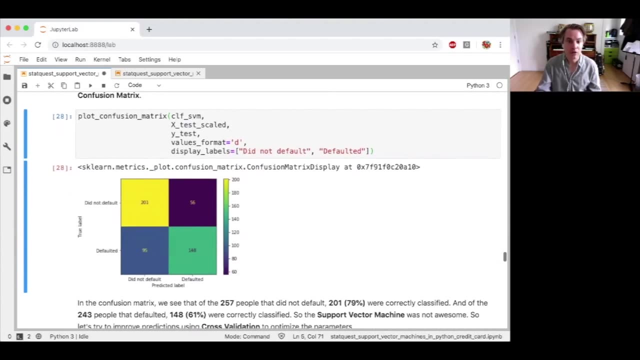 We're using plot confusion matrix. We're passing in our trained support vector machine And we're passing in the test X data set and the test Y And below we're just formatting it so it looks pretty. So here is our confusion matrix. 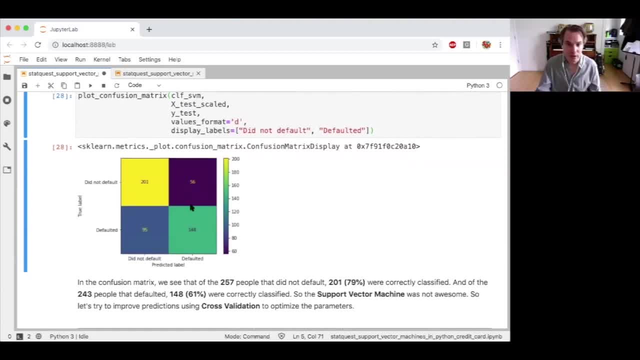 It did all right. It did not do great. Of the 257 people that did not default, 79% were correctly classified. Of the 243 people in this row that defaulted, 61% were correctly classified. So the support vector machine was not awesome. 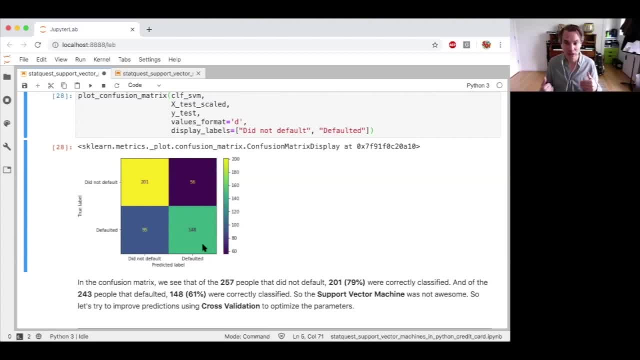 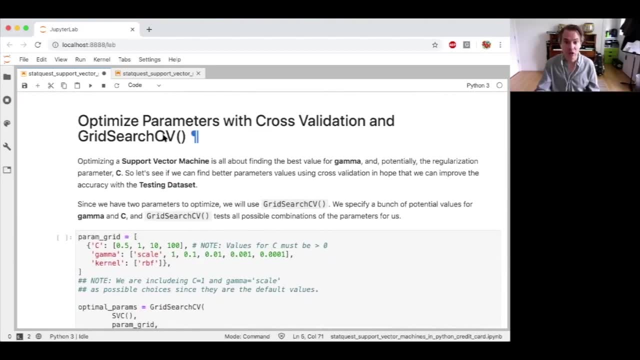 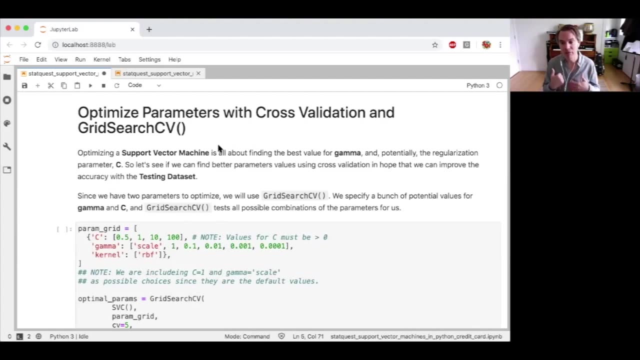 So we're going to try to improve that using cross-validation to optimize the parameters. To optimize the parameters, we're going to use grid search, cross-validation or grid search CV, And when we optimize a support vector machine, it's all about finding the best value. 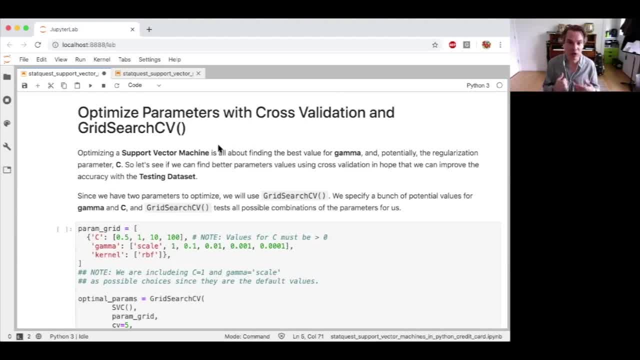 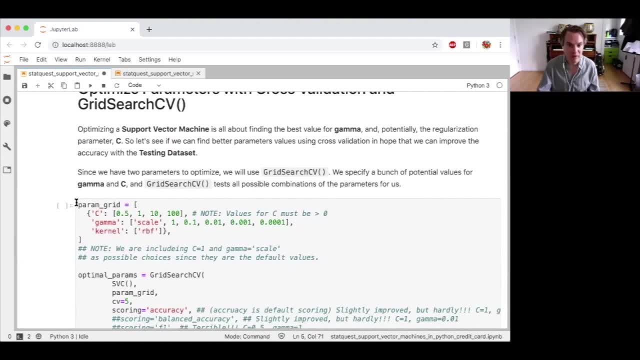 for gamma and potentially the regularization parameter C. So what we're going to do is, when we use grid search CV, we specify the parameters that we want to try in a matrix, And so we've got this is the parameter C, which is the regularization parameter. 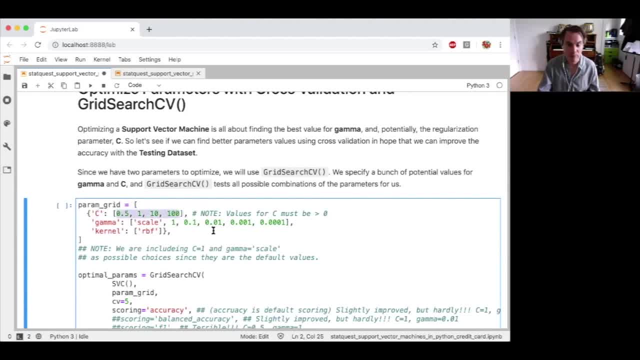 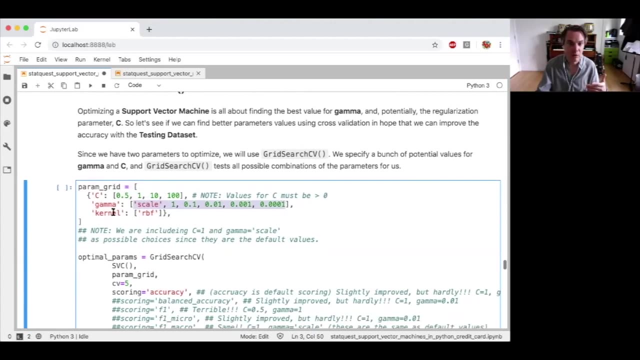 And we're going to try these values. Note: The regularization parameter has got to be greater than zero. And there's gamma, And these are the values we're specifying for gamma. In theory, we could try other kernels if we wanted to and specify those as well. 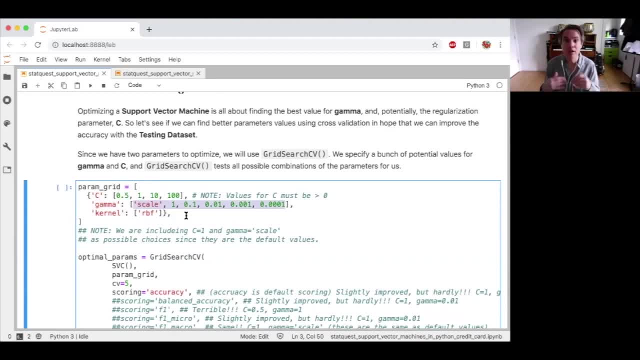 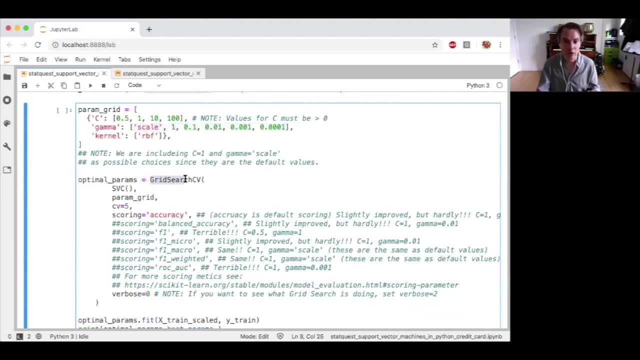 That ends up taking a long time. So we're just going to stick with the radial basis function, because typically it gives us the best performance. Okay, So then we run grid search CV And we pass in the shell of a support vector classifier. 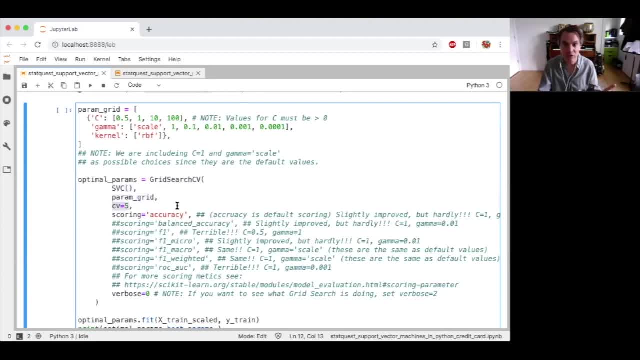 We pass in the parameters. The CV is the number of folds across cross-validation we want to do. Then we pass in the scoring metric that we want to use. There are lots of options And I tried a bunch of them. And true to its word, 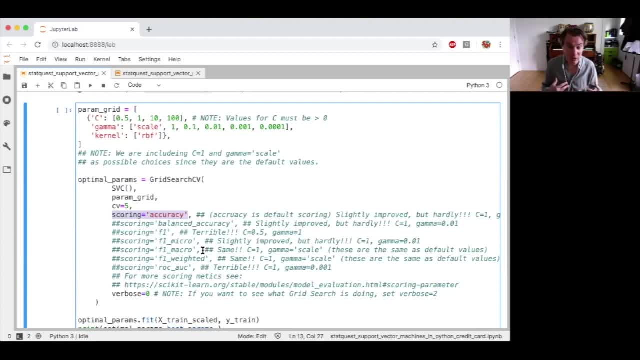 support. vector machines tend to be good out of the box And I was trying to find a metric that would give us huge improvements, And I wasn't able to find one. But you can uncomment these and try different metrics. There's even more than I'm using here. 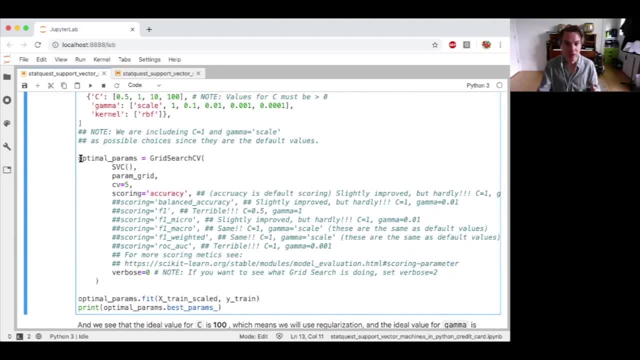 Anyways, this will return something we're saving in a variable called optimal parameters, And then what we do is we run the cross-validation on the parameter values by running optimalvaluesfit using the training data set, And then we're going to print out the optimal values. 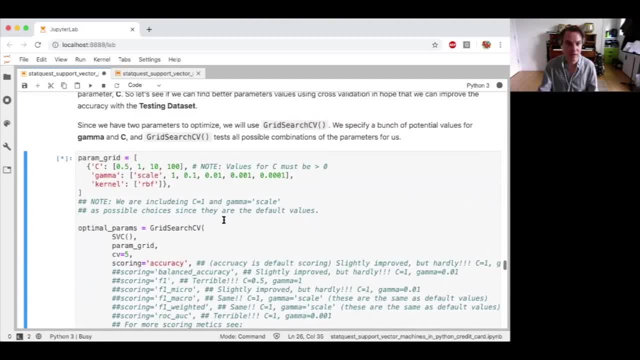 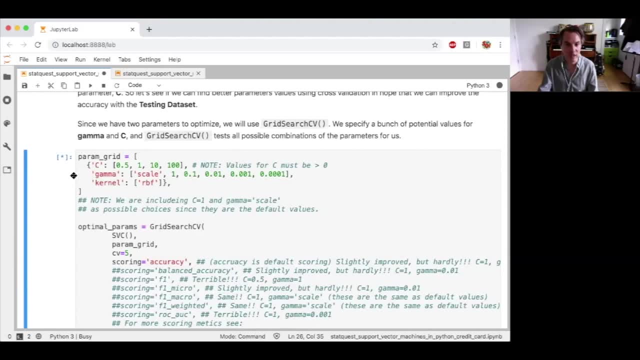 And then we're going to print out the optimal best parameters. So we'll do that. This is going to take a little long. You'll see there's a star here. That means a Python is hard at work doing cross-validation for us. 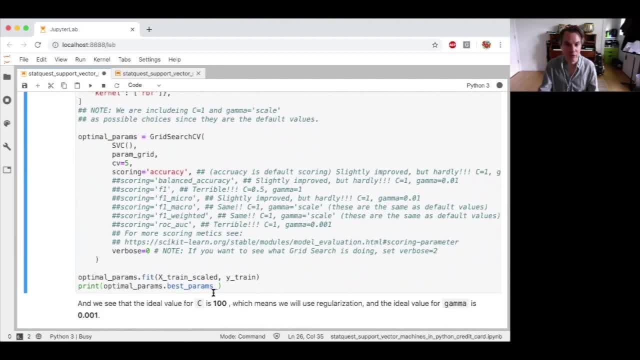 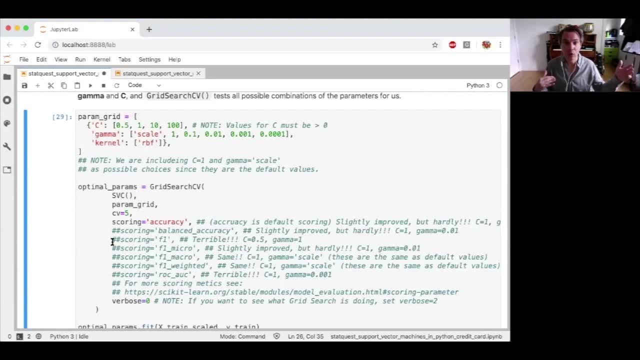 When that turns into a number, it'll print out the output down here, And this is one of the reasons why we downscaled the data set. We went from 30,000 rows to just 2,000. And it still took a little bit of time. 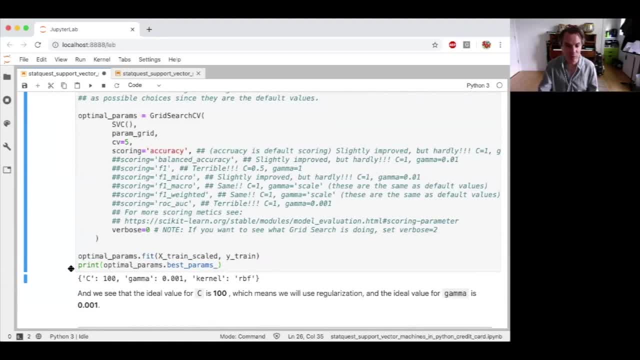 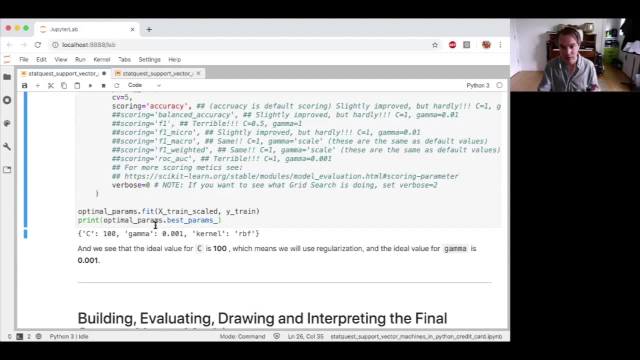 But it still took a little bit of time. These are the optimal parameters. by the way, We're done running. We've got a number here And we can see that the ideal value for C- because that's alliteration- is 100,. 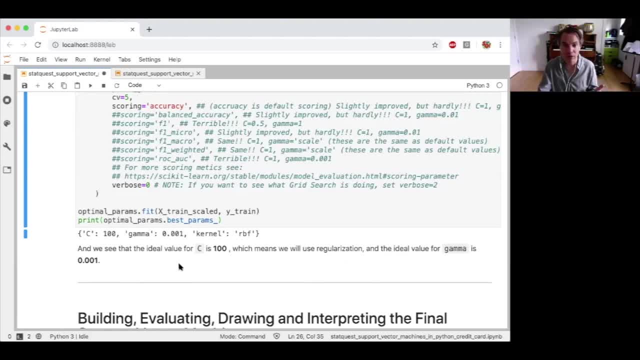 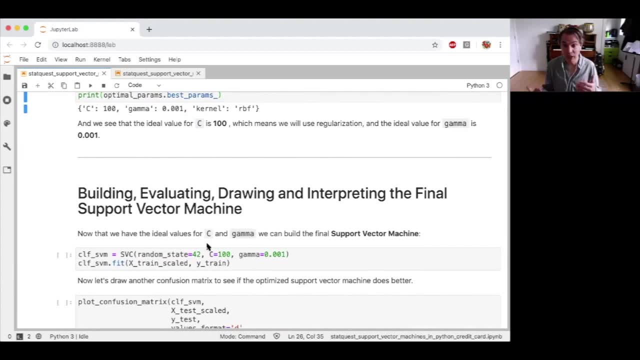 which means that we will use regularization And the ideal value for gamma is 0.001.. So now we're ready to build, evaluate, draw and interpret the final support vector machine. And now we're doing exactly what we did before. 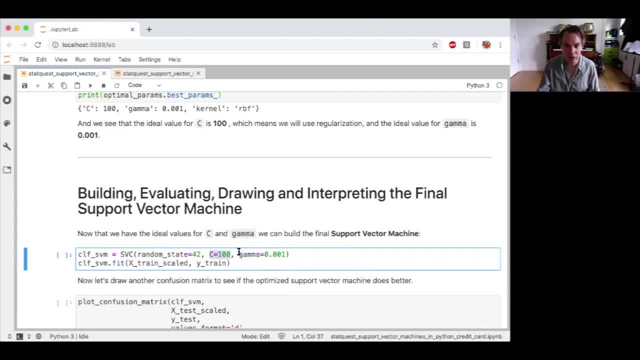 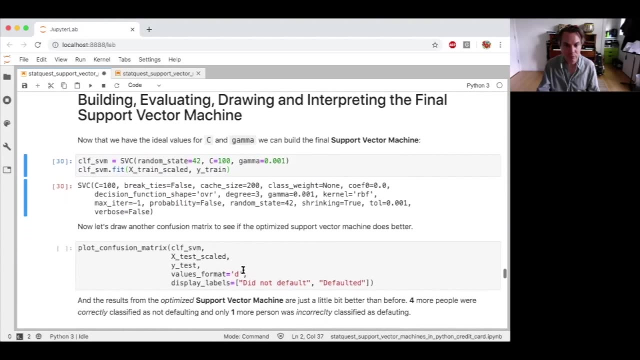 However, this time we're specifying: C equals 100 and gamma equals 0.001.. So that creates the shell, And then we train it using the training data. So we'll run that Bam, And now we're going to print out a new confusion matrix. 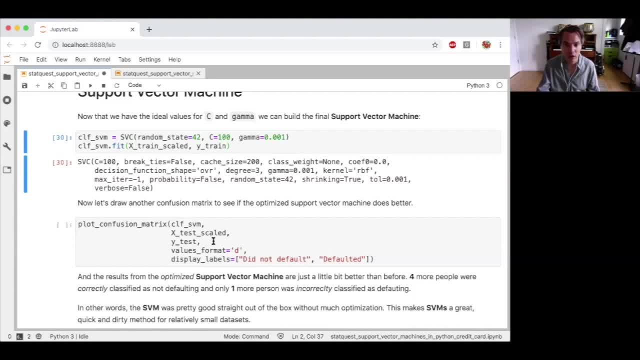 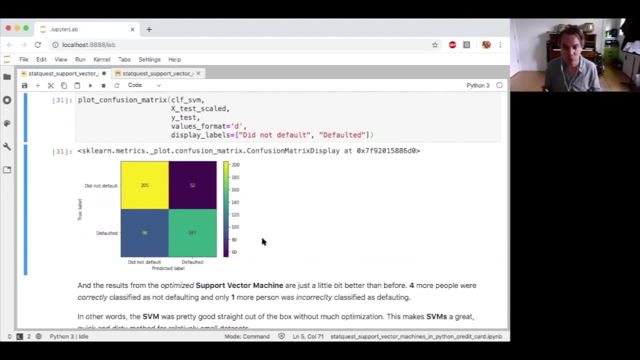 with our new support vector machine And we're going to run that And here is our output And these are the results of the optimized support vector machine And they are just a little bit better than before. Four more people were correctly classified as not defaulting. 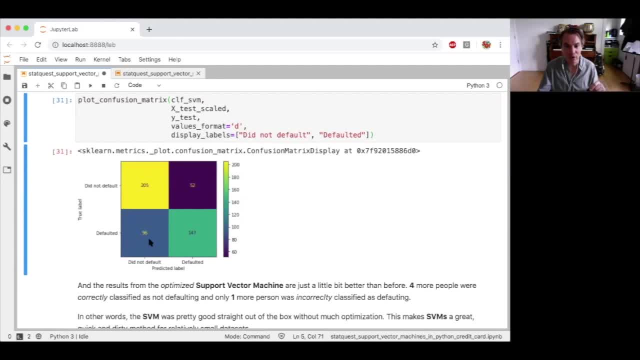 However, one person was incorrectly classified as defaulting. So, depending on whether or not it's more important to classify these people or these people, we may have improved or we may have slightly got there. We may have slightly gotten worse, But that just tells you again. 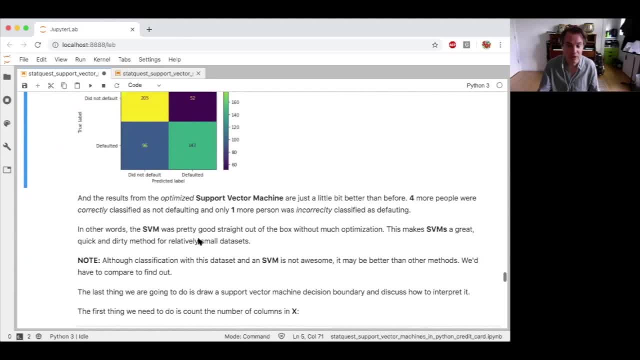 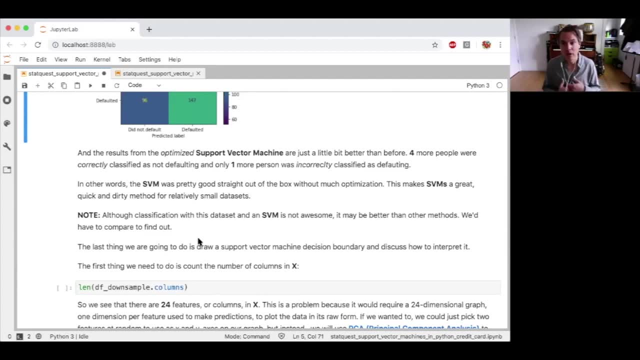 that support vector machines are pretty good out of the box Optimization didn't help us that much. OK, Now we can actually draw what the decision boundary is. This is a pretty complicated procedure And at best it is an approximation of what is really going on. 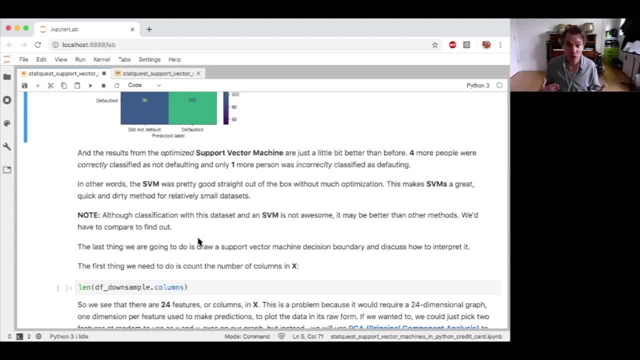 And we can quantify how good that approximation is. There's various ways that we can quantify how good that approximation is going to be, And we'll go over that really quickly. The first thing we're going to do, though, is we're going to look and see how many columns 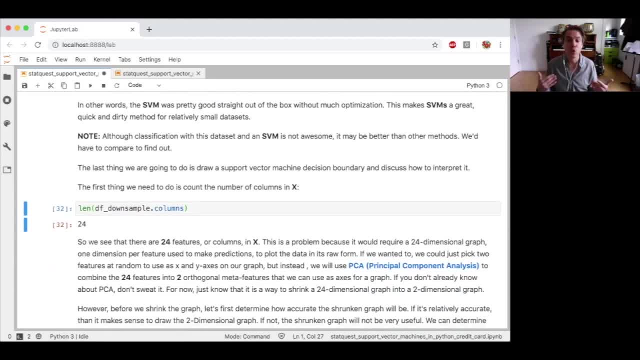 in our data set. So we've got 24 columns in our data set And this is a problem, because that means it would require a 24-dimensional graph, Or maybe even more, because we're using the radial basis function And that operates in infinite dimensions. 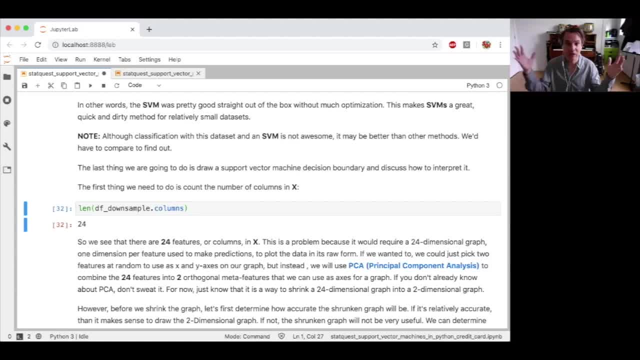 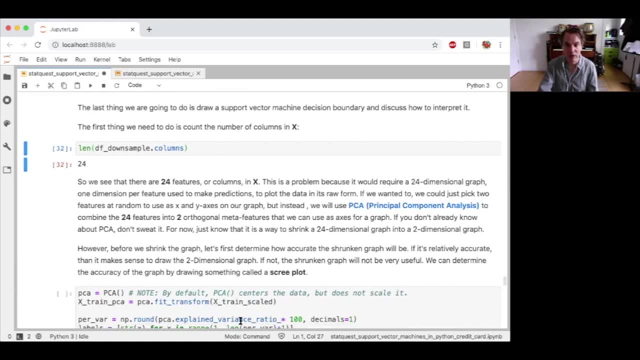 And since we can't draw an infinite dimension, we have to do data, We have to collapse the data into two dimensions so we can draw a picture of that. We're going to use principal component analysis to do that, And if you don't know what, principal component analysis? 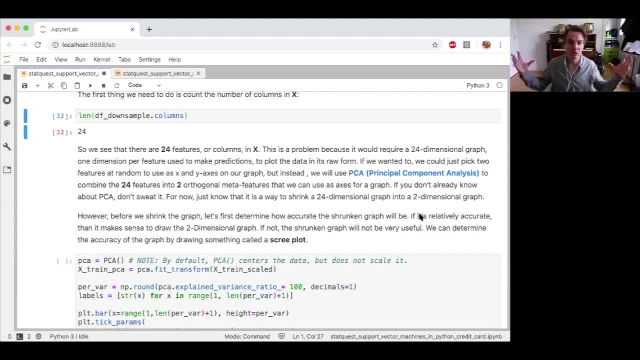 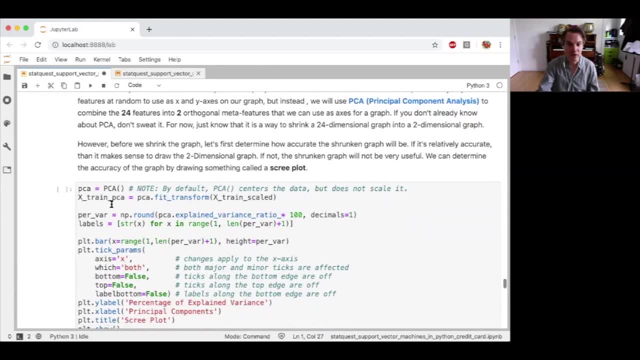 is right now. just know that what we're doing is we're taking those 24 columns and we're going to shrink them down to two. So this is the code for doing that, And we're also going to plot what's called a scree plot. 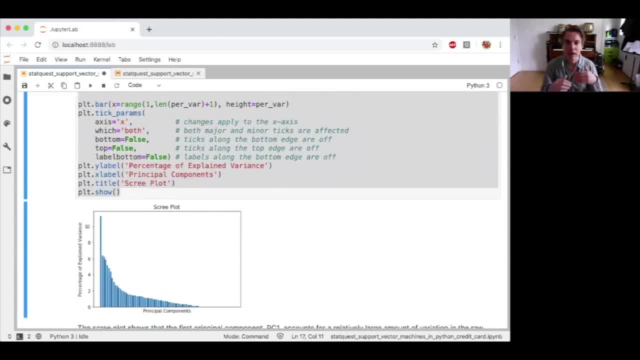 And this scree plot tells us how good this approximation of the true classifier is. What we would like is for the first two principal components, the first two columns here, to be much taller than all the rest, And that means that those first two columns 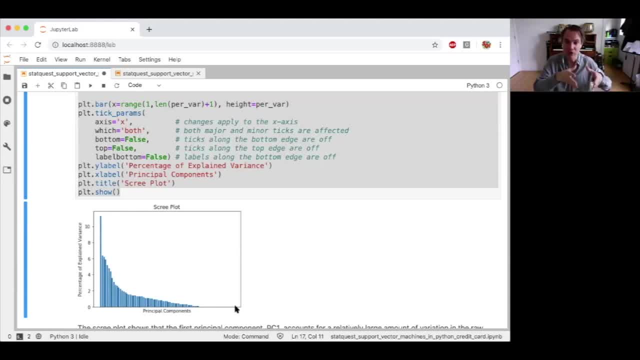 or those two columns that we're going to use for our new data set, would accurately reflect the original data. In this case, we don't see that. What we see is that the first principal component, the first column, stands on its own. That's good. That's what we want. 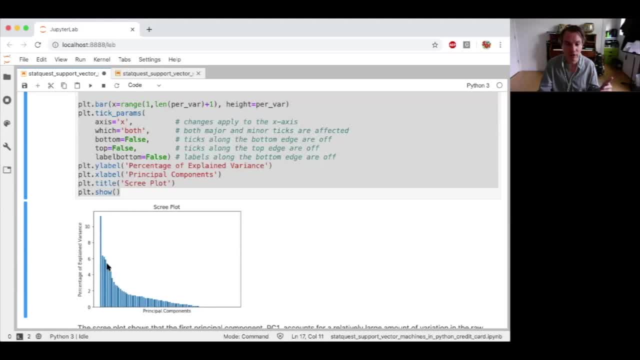 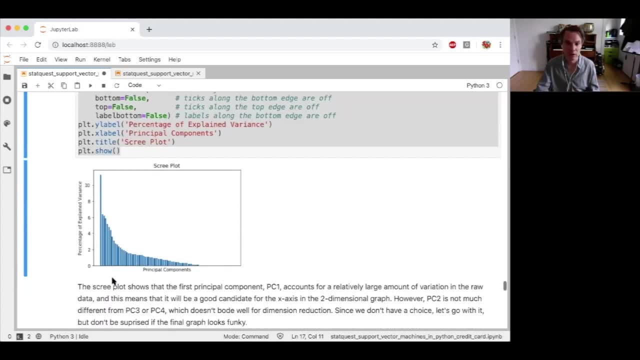 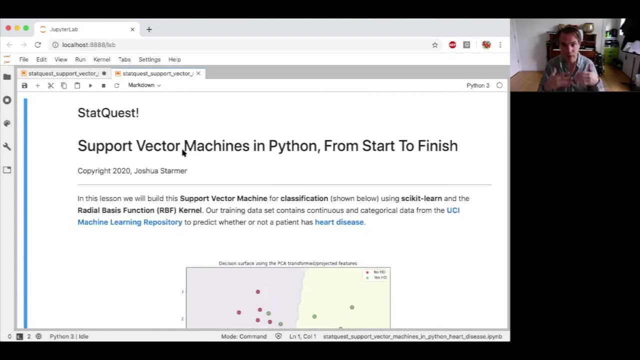 However, the second one is just barely taller than the others, and that's not good And that tells us that this approximation is not going to be great. That said, I'm also including in this in the email I'm going to send out. 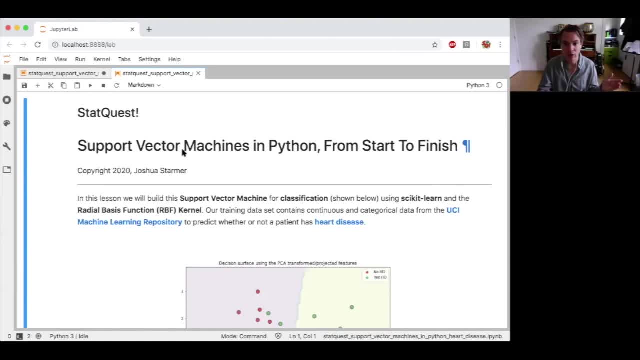 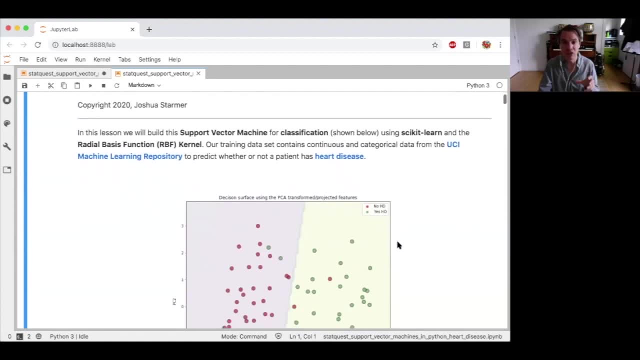 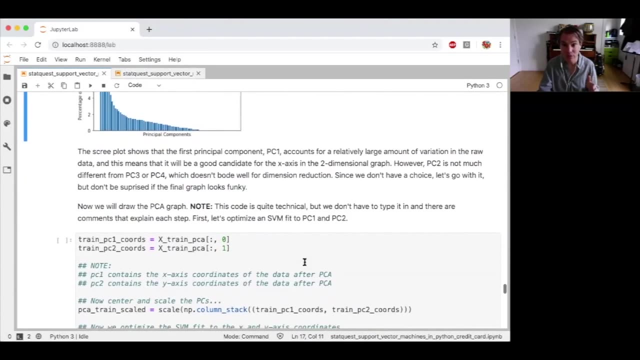 you're going to be able to download how to do support vector machines with this heart disease data set And in that case the image is better and actually classification in general is better. So make sure you run through both of these because you'll get different results. 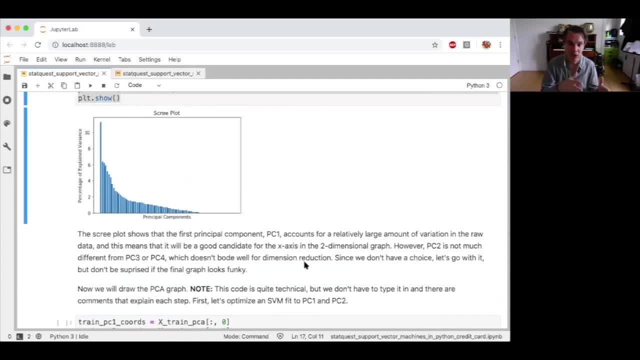 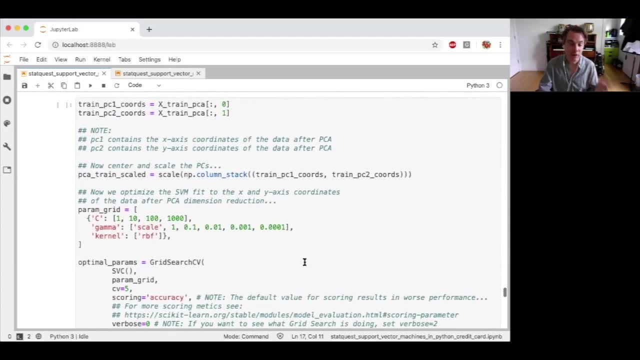 and you'll see that how to decide when it's going to be a good sort of collapsing of data and when it's not. The next data is pretty complicated. next code chunk. However, just know that what we're doing is we're retraining and re-optimizing. 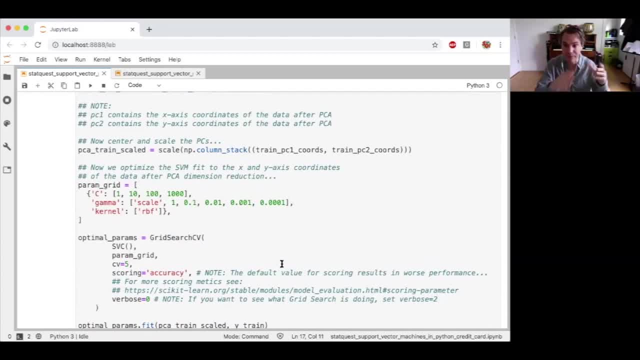 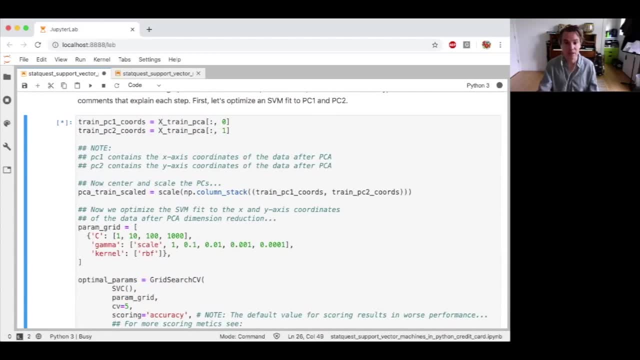 a support vector machine on just those two columns that we collapsed the data down to. We run that, We're doing cross-validation, so this is going to take a minute or two And while this is running I will address this one question. 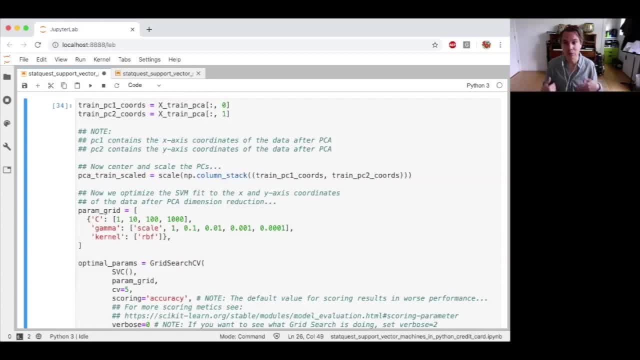 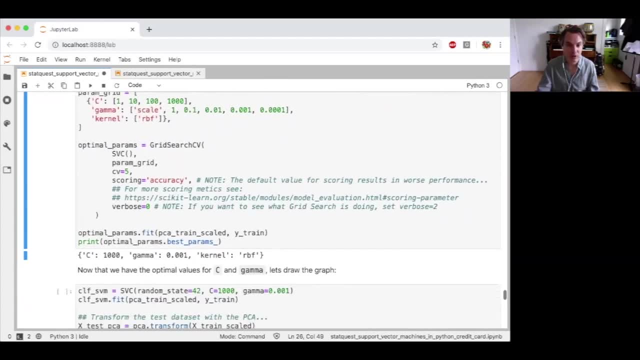 Yes, we are recording this as a video and I'll put it online and you'll be able to access this later on at your leisure and I'll email you the link. Okay, so it's done running. We've got optimal parameters. 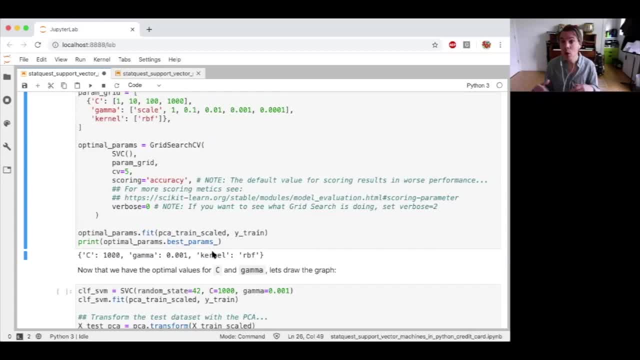 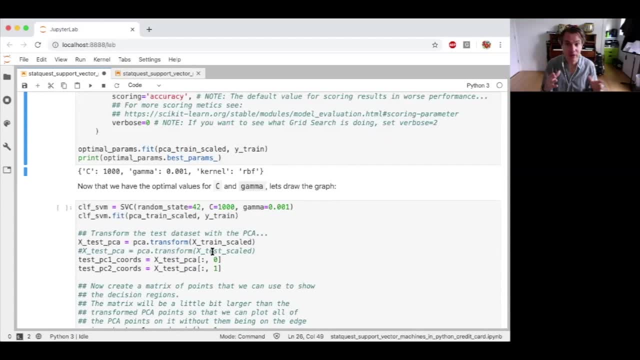 Notice we've got different optimal parameters than before. That's because we're actually using a different data set. Instead of all 24 columns, we're just using two now, And that's you know. like I said, we're approximating what we did with the 24.. 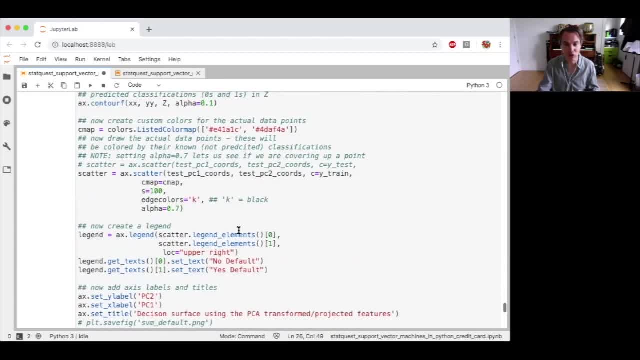 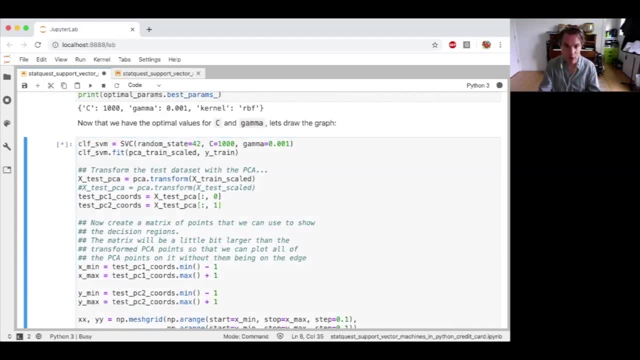 Here. this is when we're actually drawing that decision: boundary. Lots of code, but also very well commented, So you can go through this at your leisure. Right now, we're just going to run it really quickly and we're going to look at our picture. 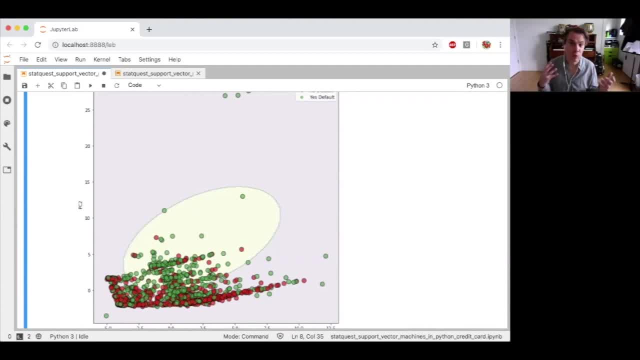 and here it is Kind of a mess, but kind of what we expected, because the first two principal components, which form the X and Y axis of this graph, don't do a great job capturing sort of all the variables and the variation that's in the data.